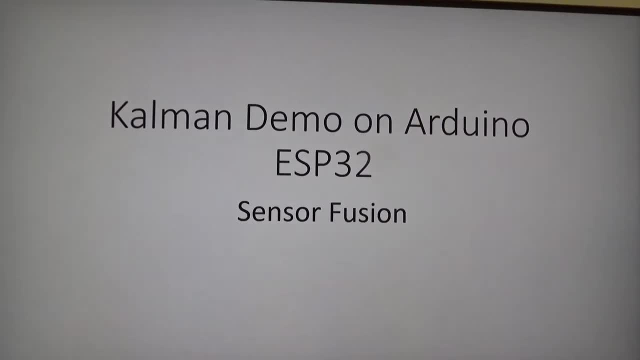 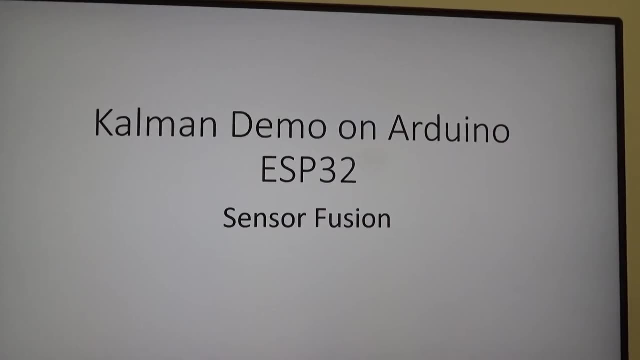 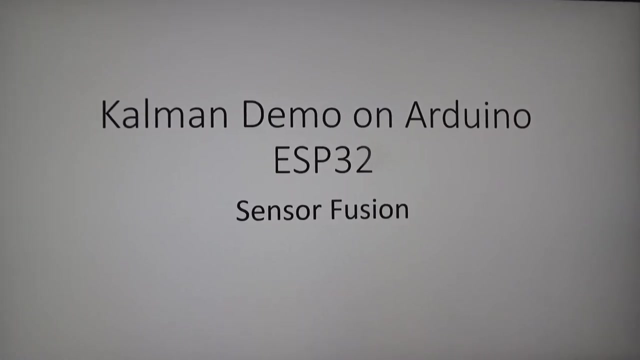 Welcome back. Today I'm going to be looking at Kalman Filter again. It's a real-time Kalman Filter demo, but this time on the ESP32, using the Arduino language. We could, of course, use Python or some other language. We're going to use what's called sensor fusion. I'll explain. 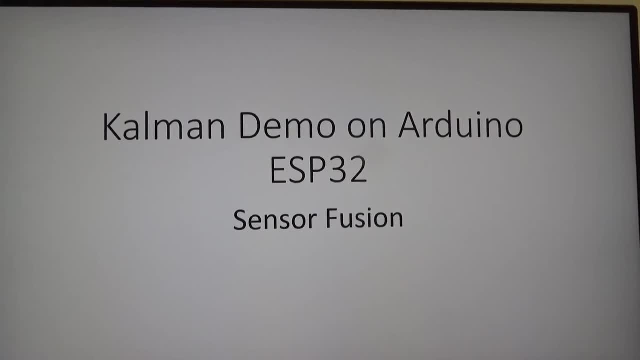 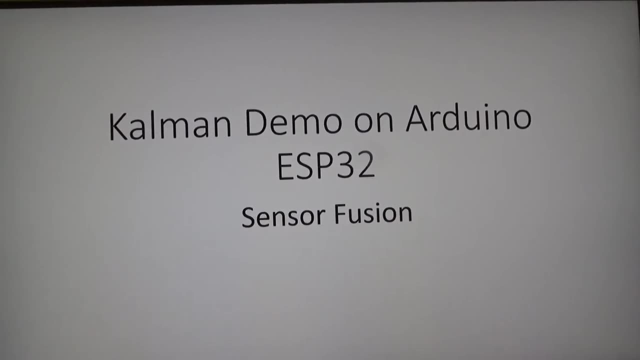 that in a minute. So this is the sort of thing that if you're trying to measure the tilt angle of something- maybe for a quadcopter or a sedgeway- you're trying to keep the thing balanced. It's like a balancing exercise, Or it could be for an aircraft or whatever, but 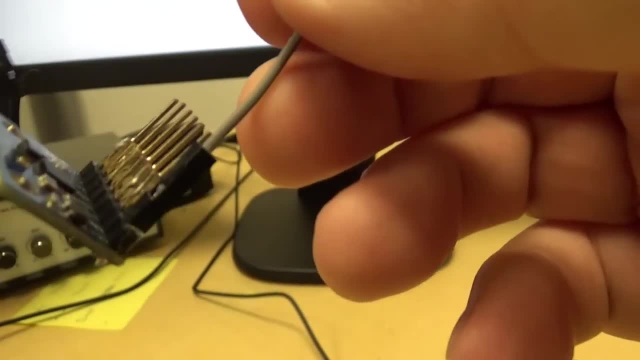 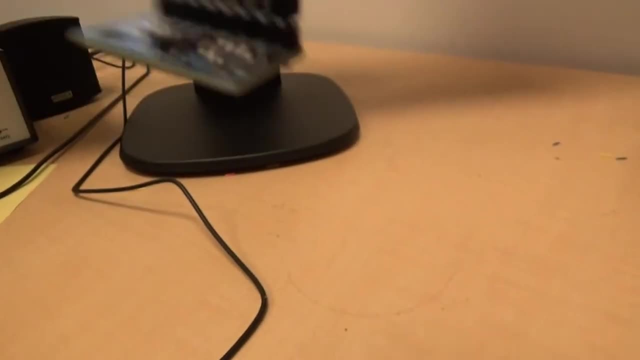 not for this particular device. This is the MPU6050, which I'm sure a lot of you have seen. This is the actual chips on here. This is a board that you can buy, which is already made up, so you don't have to do too much. 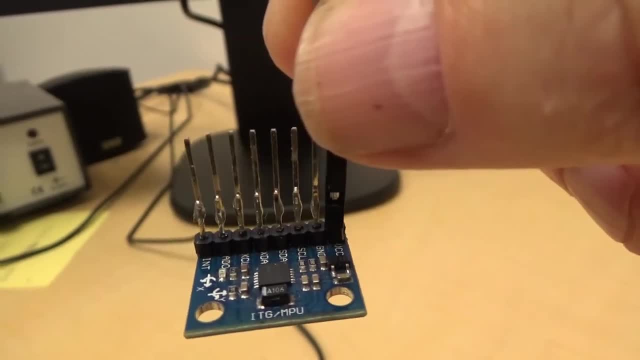 and you only need a few chips, So you don't have to do too much. and you only need a few chips. So you don't have to do too much and you only need a few chips. need about four of the pins there. One's off 3.3 volts. sell for a couple of. 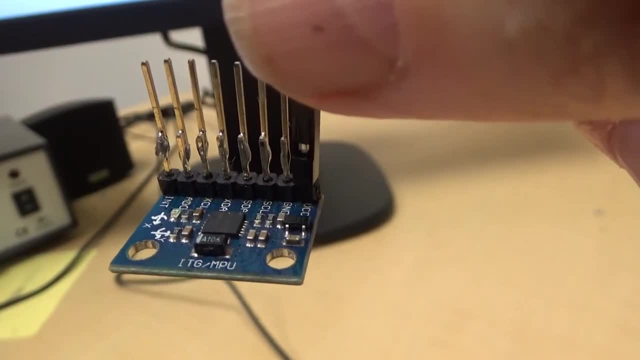 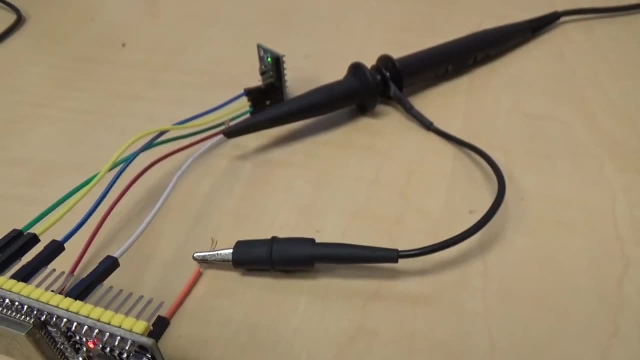 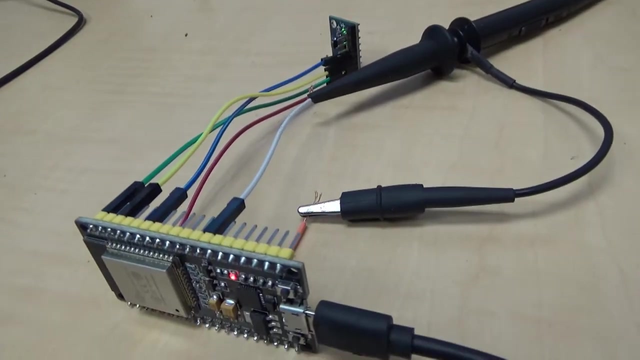 dollars and that's going to be connected to the ESP32.. So I've done that over here and it's just only connected through the I2C. I believe that's the Philips interface, This is the ESP32 and that's the MPU6050. 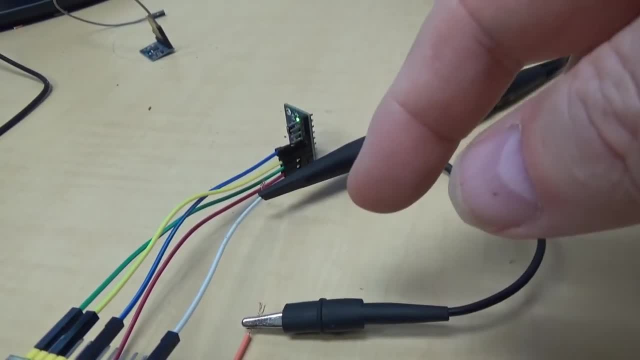 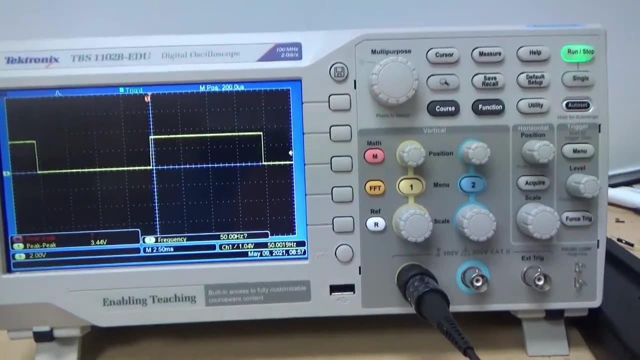 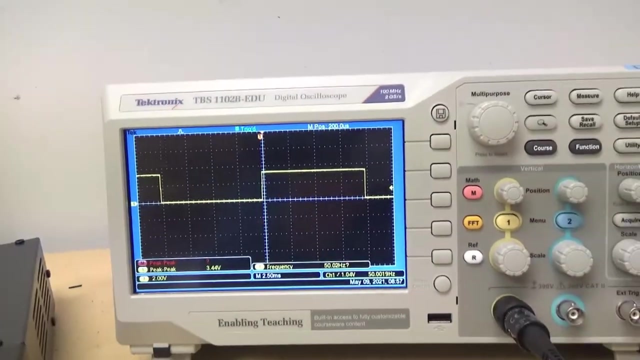 I've got the oscilloscope leads running off it and I'll explain in a minute. but basically the scope here is just a waveform and if you look at it you read what it says. there it's reading 50.00 Hertz, That's the sampling rate. 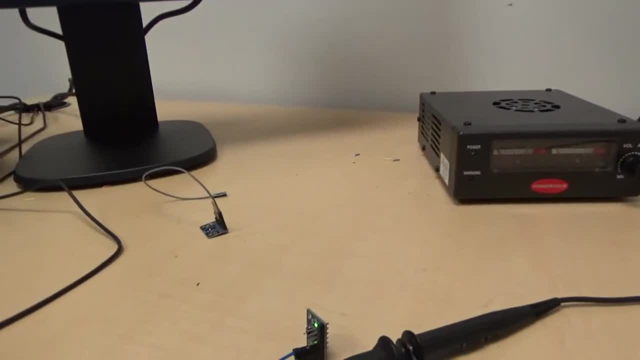 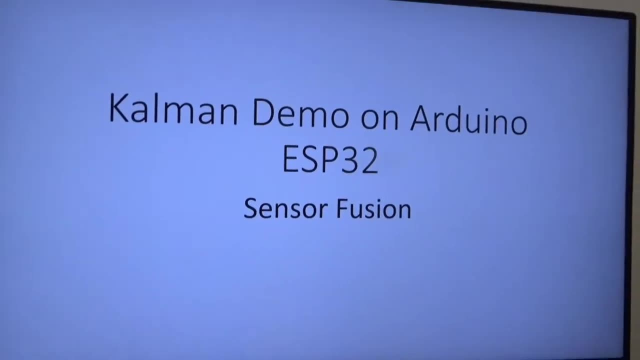 that I've set the whole thing up for to acquire the data, and that's pretty accurate. So let's just have a look at the theory first to see what we're doing Now. there is another line here. This is a lecture I've given online about the Kalman filter, which is a little bit. 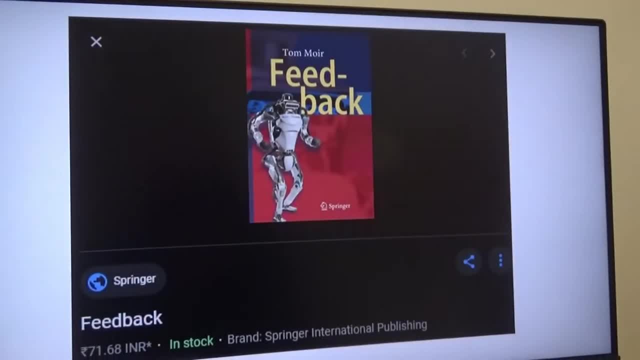 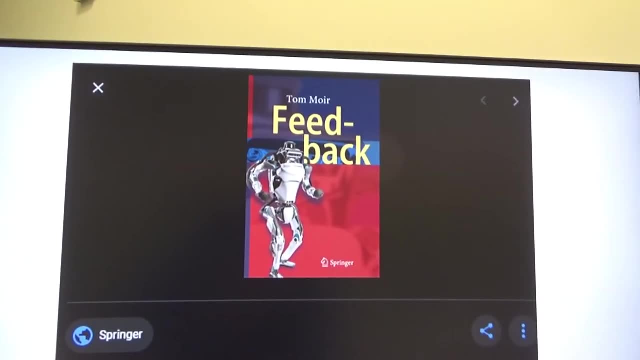 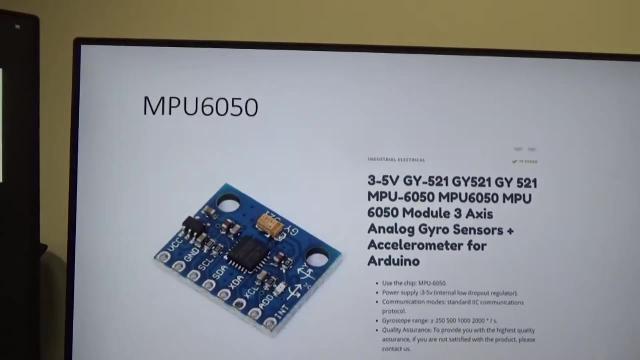 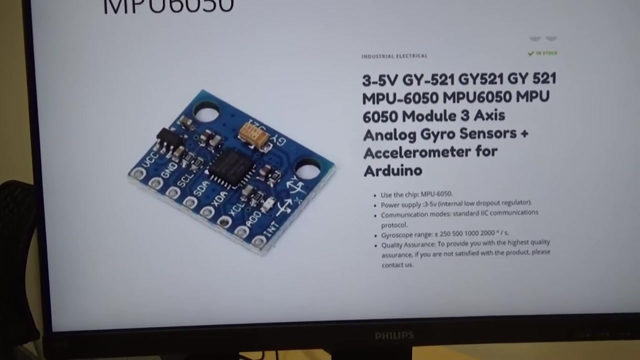 more detail. Some of this comes from my book, which was published last year, January last year, 2020.. It's called Feedback, published by Springer. So this is the MPU6050 that I've just shown you. It runs off 3.3 or 5 volts. 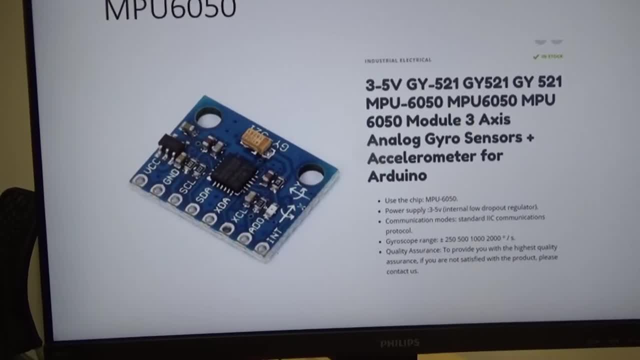 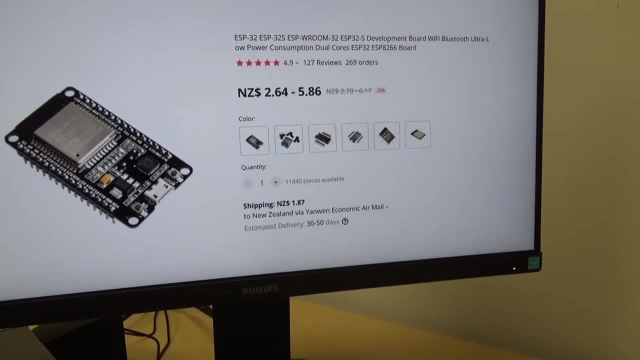 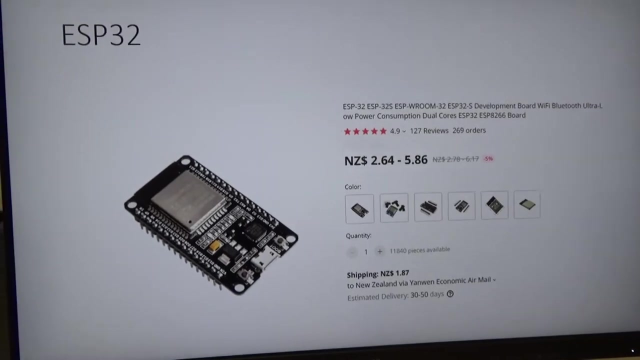 And it's very easy to connect up. There's only four pins And this is the ESP32. It's pretty cheap as well. It's New Zealand dollars, about anything up to six dollars New Zealand. It's only a few US dollars, depending on the quantity you 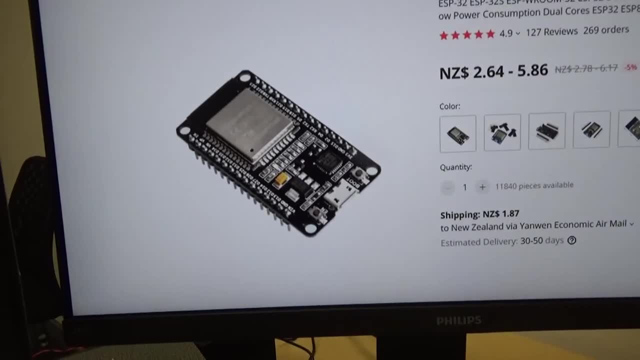 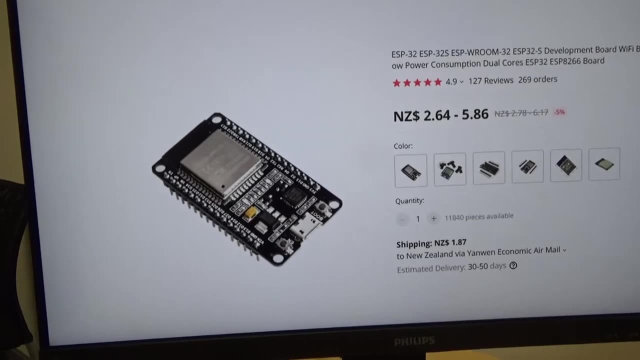 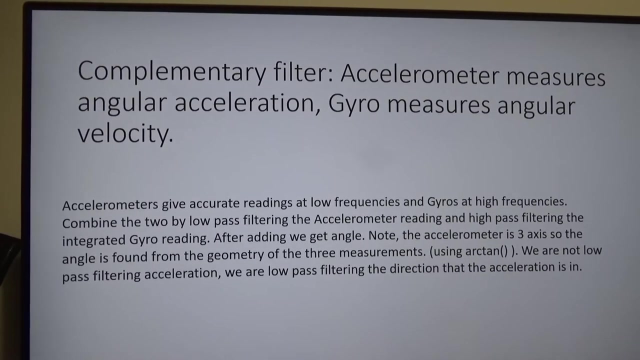 buy them in. They come in different number of pins. This board, the actual device itself, is here and these are just a little board that it comes with. It's a little board that it comes with. If you need that, it's handy to use that. So what this small device here gives us. 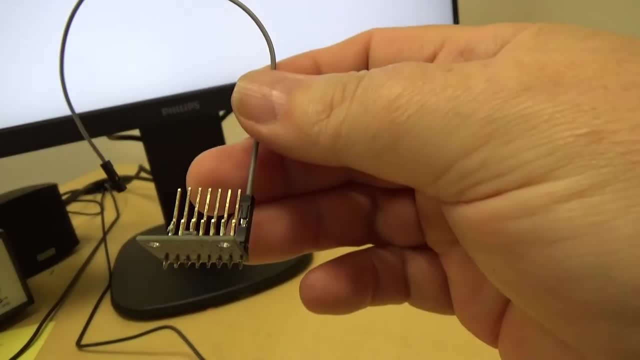 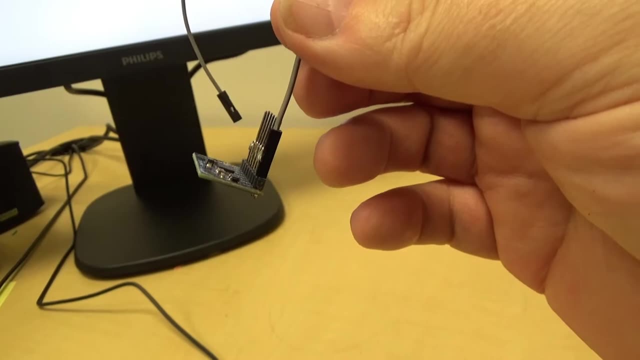 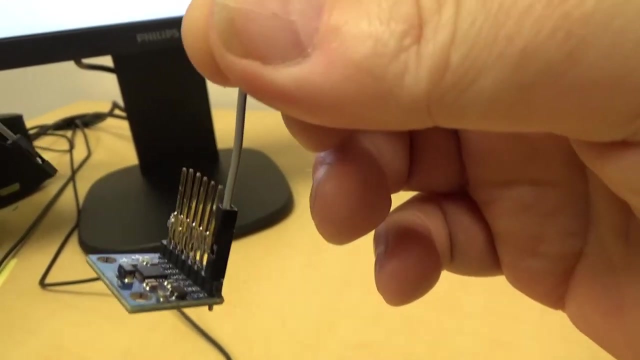 is. it gives us 3-axis acceleration and 3-axis velocity from a gyro, So the gyro gives velocity and acceleration comes from accelerometers. It's in 3-axis though, so we've got to be careful how we get this and how I 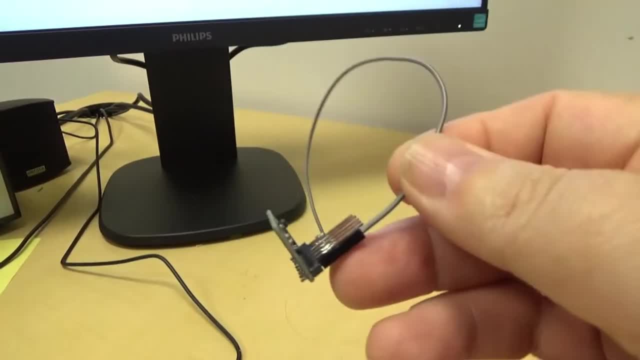 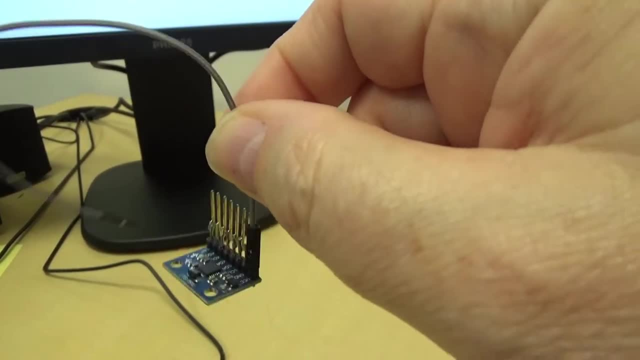 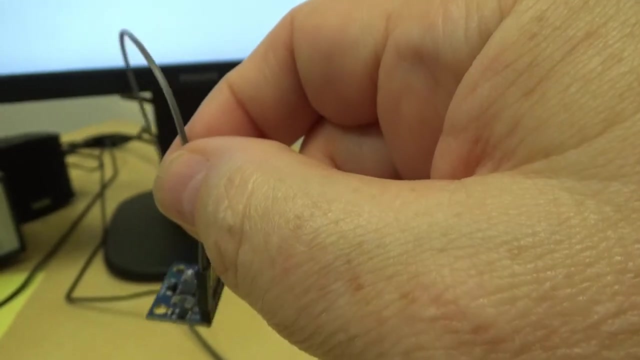 define this here is that this is pitch that angle and this is roll okay, in that direction. This would be yaw, but unfortunately it can't work out. yaw, You need a compass for that. Yes, I see a lot of people trying to do this online, but you. 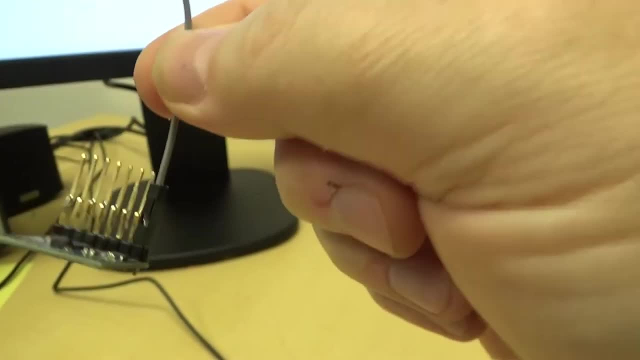 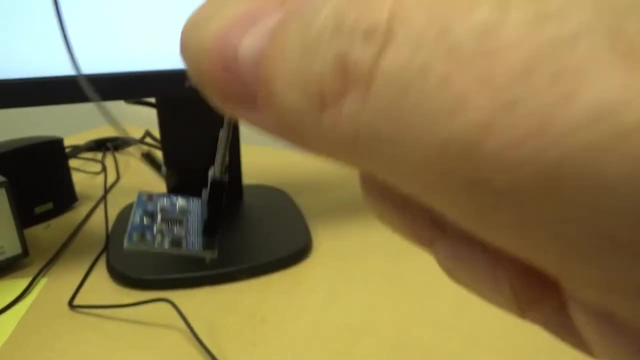 you can't do it without an extra different chip. There's a more sophisticated one that has got a compass, and then you have to set that up in a special way. This one hasn't got the compass, so we can only do pitch and roll. I'm only going. 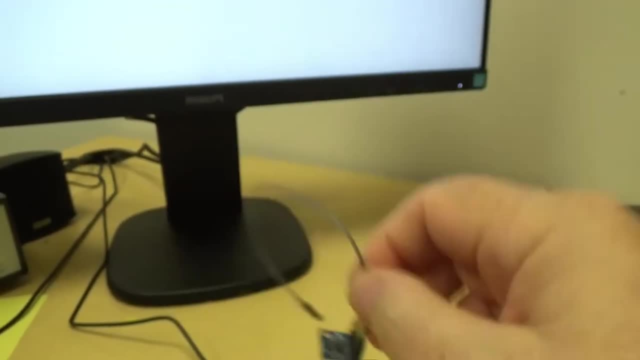 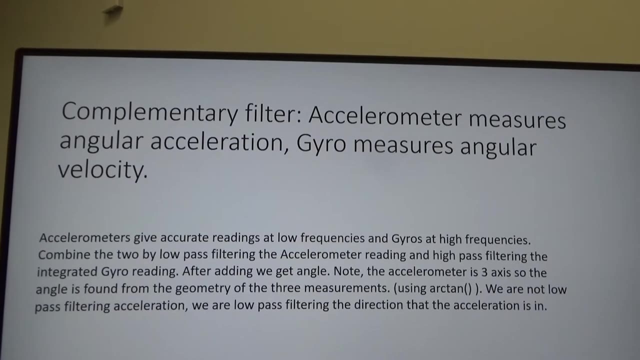 to do. pitch here, though, however, to give you an example of how a Kalman filter works, But there is another way you can use other than a Kalman filter. you can use what's called a complementary filter, which I have used in the past, and it's 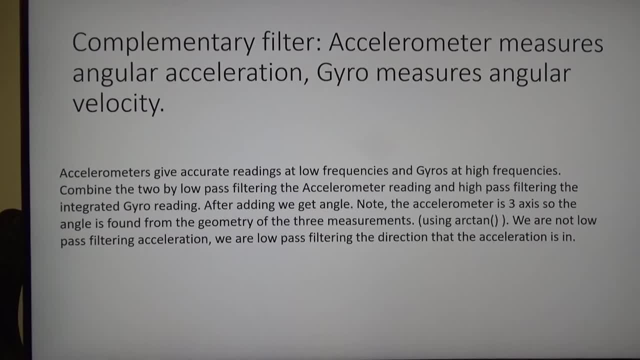 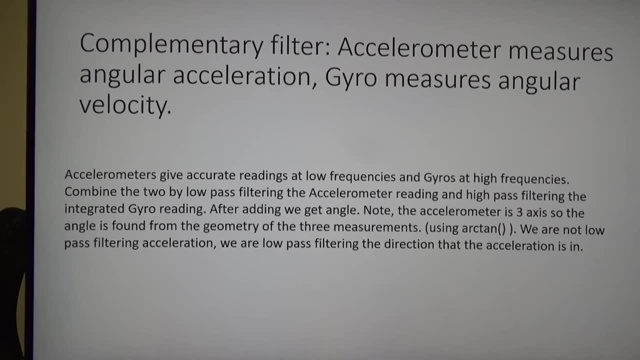 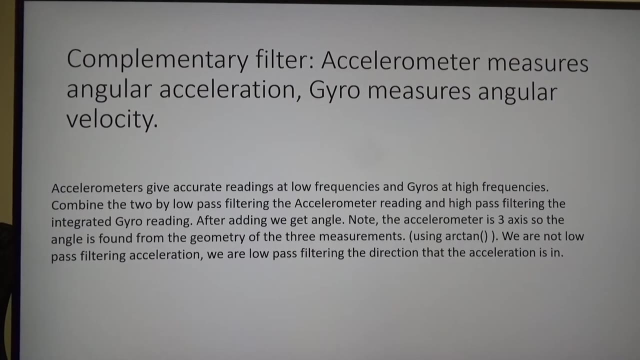 because accelerometers give accurate readings at low frequencies and gyros at high frequencies. There's a necessity really to combine the two so that you get the best of both worlds. We can, of course, just use accelerometer readings and I can show you what they look like. They're okay, but a little. 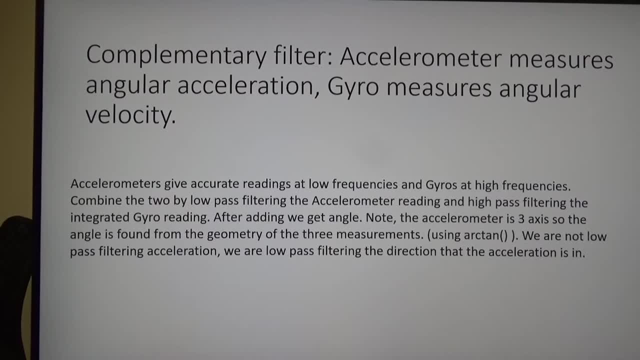 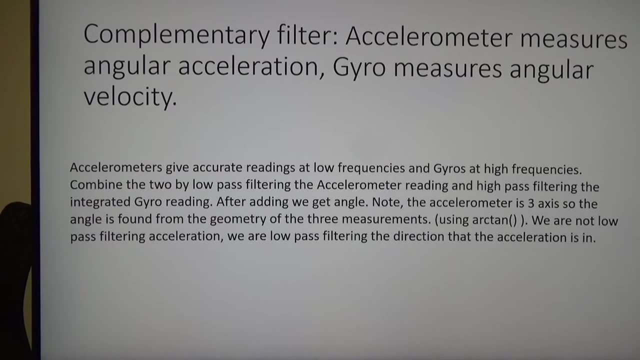 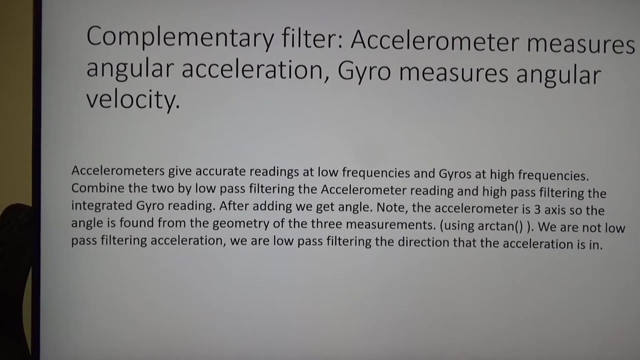 bit noisy and a bit sensitive too, too sensitive if anything. Whereas accelerometer- sorry, the gyro readings- will give you angular velocity. So to get to position from velocity you need to integrate the gyro reading. Now, integrating anything is a bit of a pain. 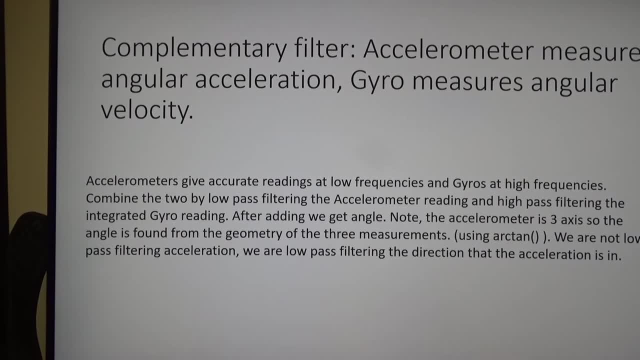 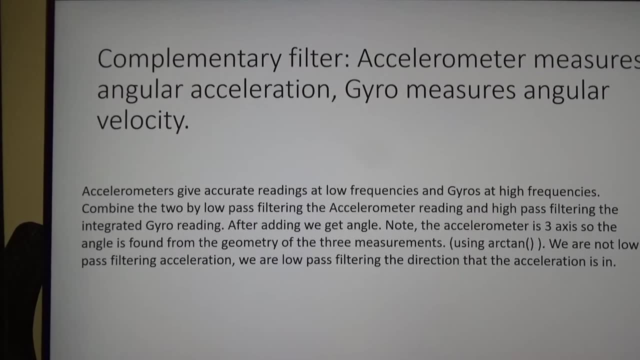 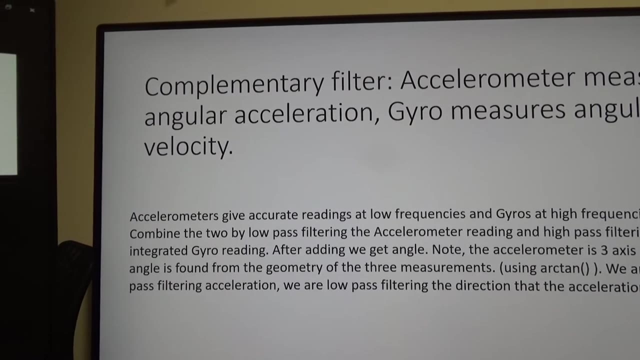 because certainly in an open loop system, because any a small amount of DC that gets into it and it just gives you huge errors. So integration, an open loop form, isn't good. Likewise, if you had acceleration in you wanted position, you might think I just need to accelerate to integrate. 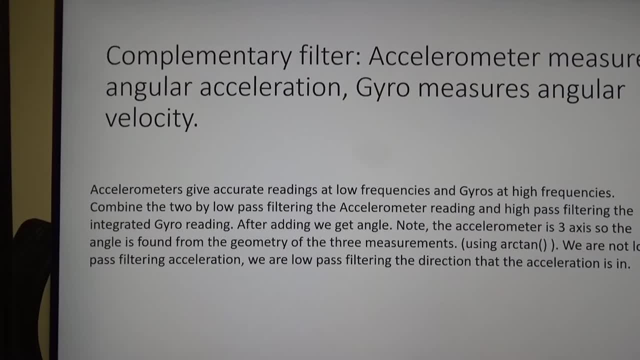 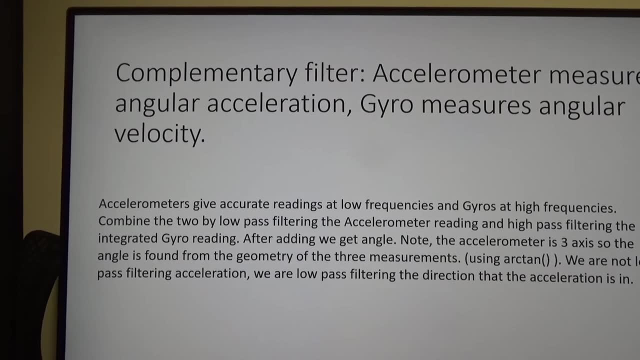 twice. But again, that's even worse still. But we don't actually have to integrate our accelerometer readings when you, when you think of it, or the confusing thing is, when you look at the accelerometer, you think I need to accept to integrate it twice to get position, but you don't. 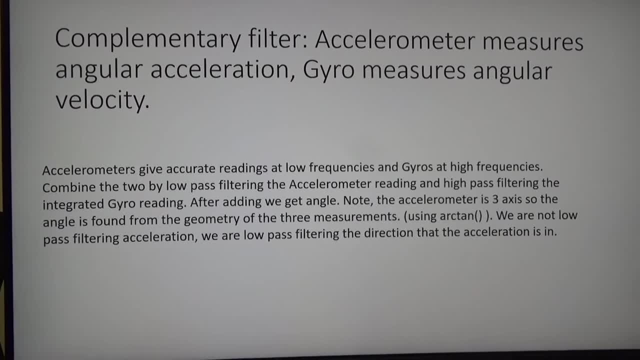 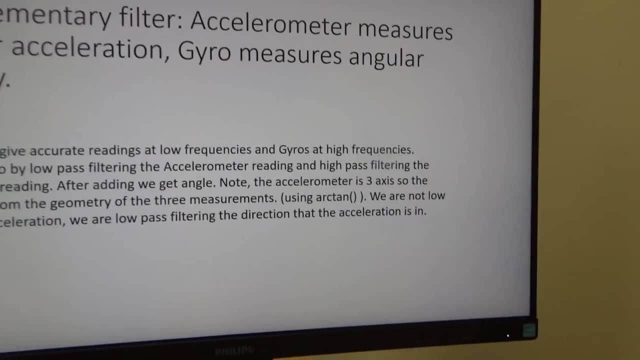 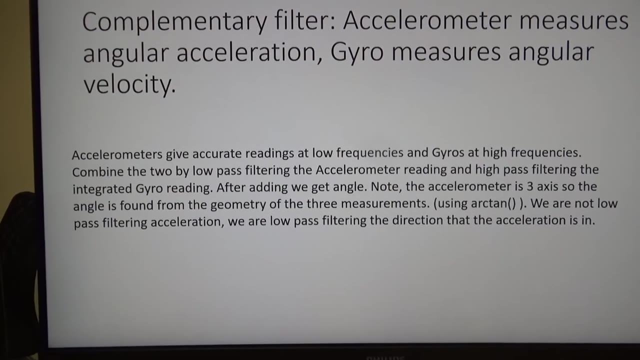 actually because it's the direction that the accelerations going in, that we actually use and we use the arctan function for this. so if you low pass one of them, they see the accelerometer one it's got to be, and you high pass the other one, because it's that's the gyro. one is good at high frequencies and then 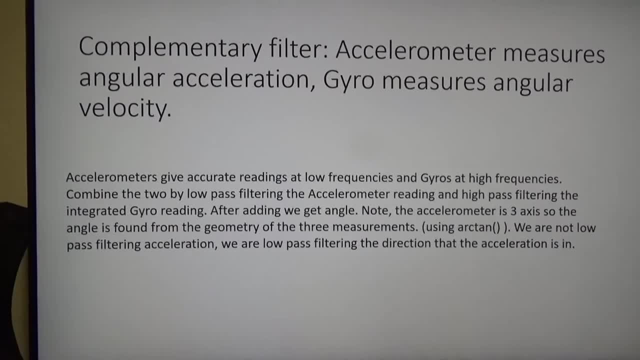 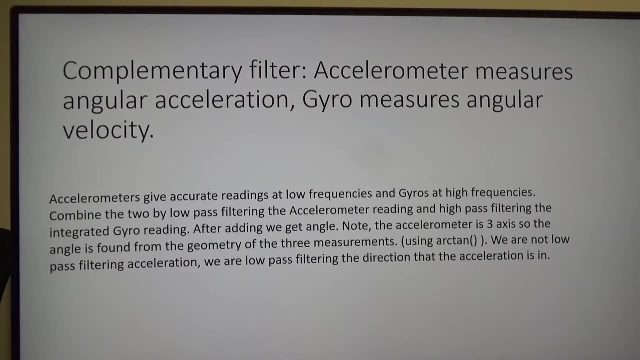 you combine the two, you basically just add them. it means that the filters got to sort of add up to one when you you know the low pass and the high pass one, and it's a very simple way of doing it and there is a some kind of success in. 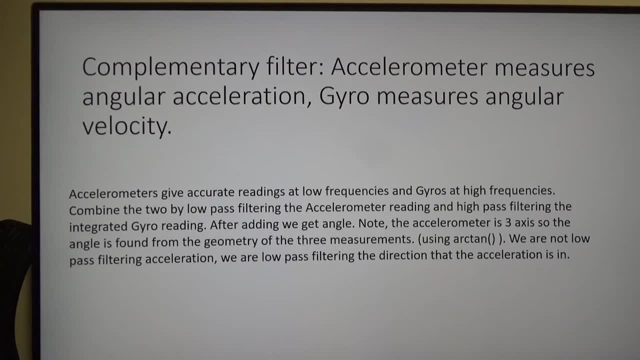 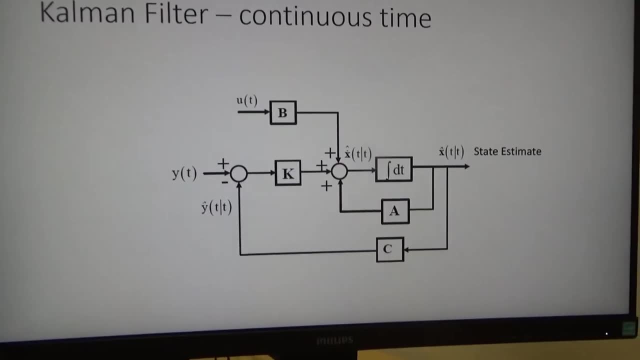 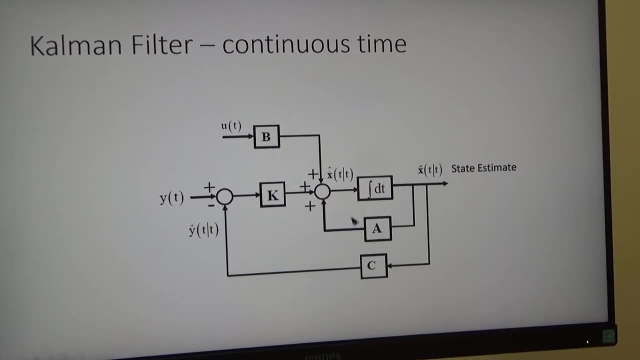 doing it that way, but it's not the method I'm going to use here. instead, I'm going to use a common filter. it's a little bit more scientific. this is the block down of a calm block diagonal of a continuous time common filter. it's got feedback around it. you. 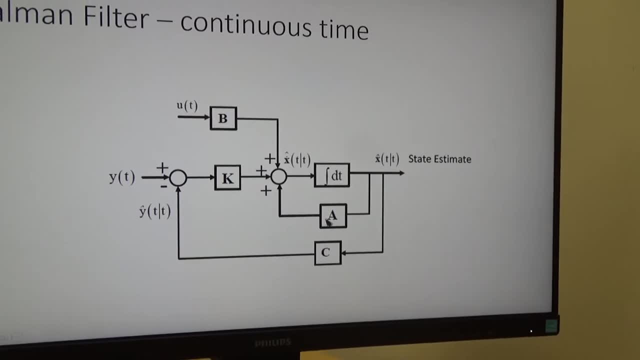 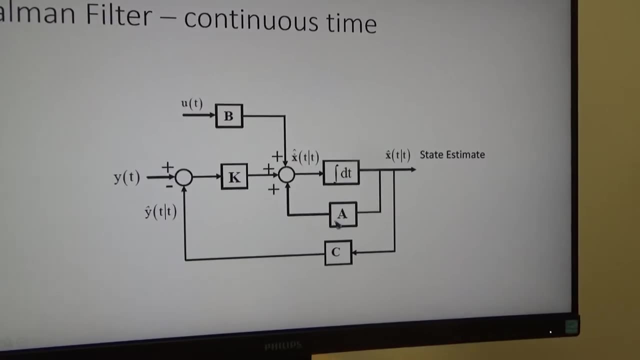 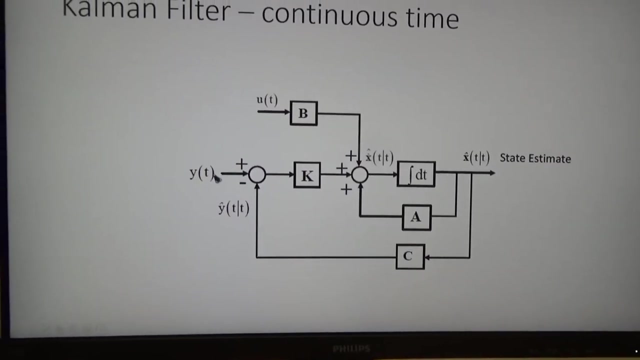 should understand state space in order to understand this and how systems represented in state space then integrate. so that's the, a matrix of us continuous time state space system: X, dot equals ax, was bu. y equals CX. the observations: that's the. in this case this is going to be multivariable because we've got 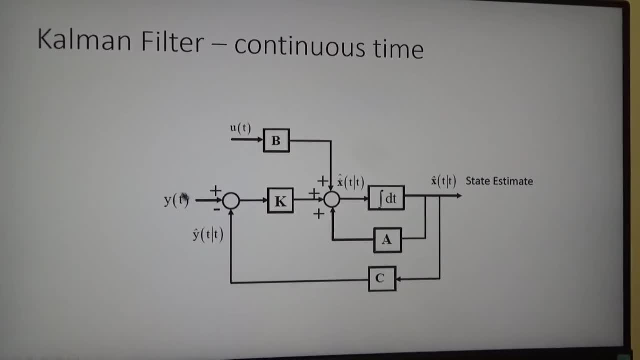 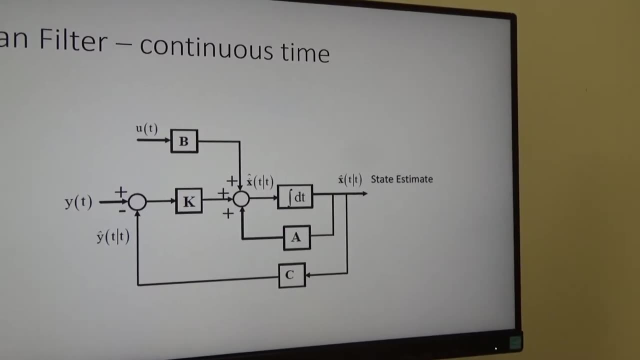 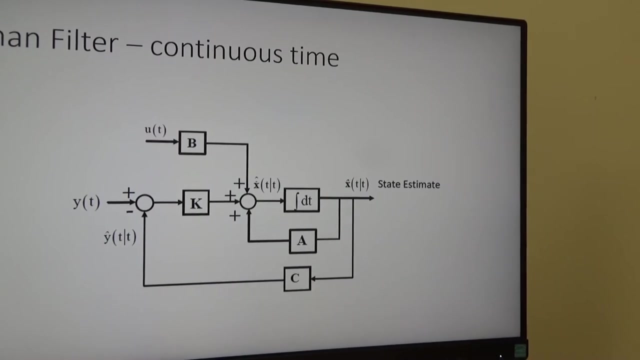 accelerometer reading and the gyro reading coming in here. so that would be actually a vector here and what we get out is a vector which is state estimates, the state estimate, and that will be position and velocity. a position of velocity actually is a good thing for control systems because a great for us. 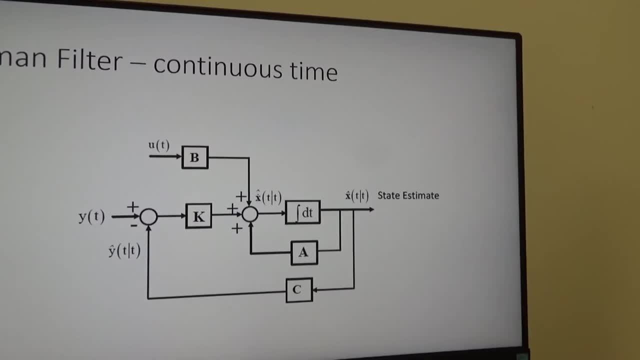 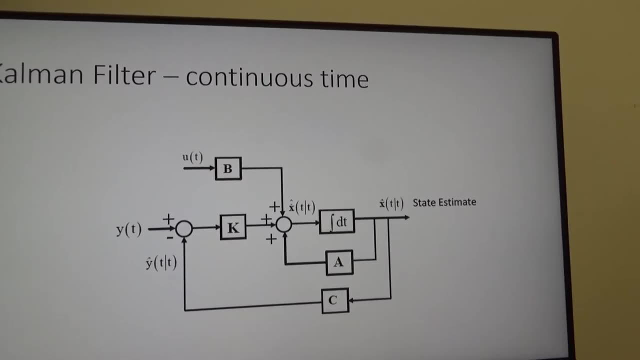 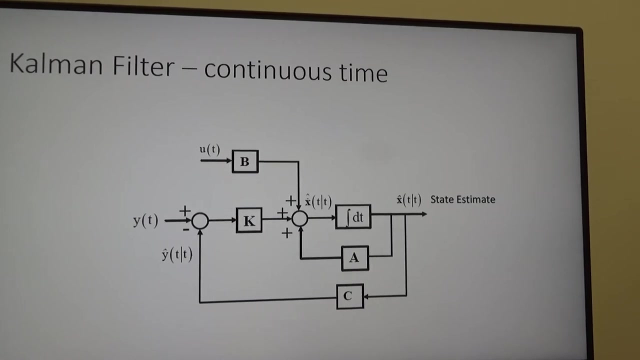 feedback. feedback position to control the tilt or whatever angle. and velocity is stabilization. it's the first derivative of position. so it's like position, it's like proportional plus derivative control of your feedback. the states when it's: you've got position and velocity. this bit, here the B term isn't 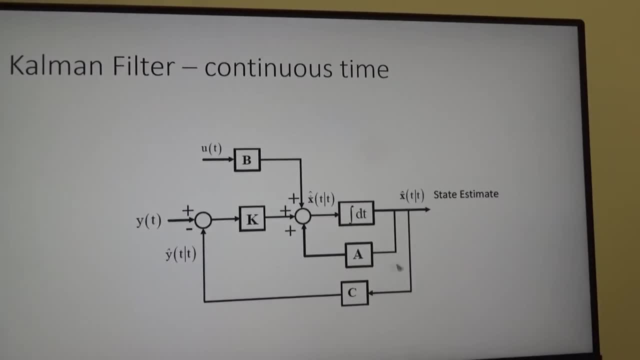 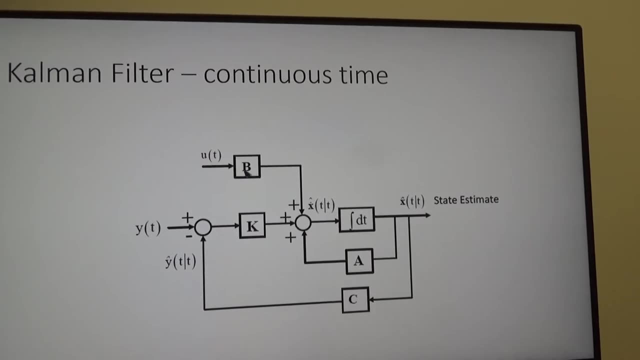 really used here at all and we're just using in the filtering mode that is in the original theory of the common. filter is needed if you're controlling something around zero, which is what I'm doing- actually not doing any control, I'm just actually doing the filtering, but that's. 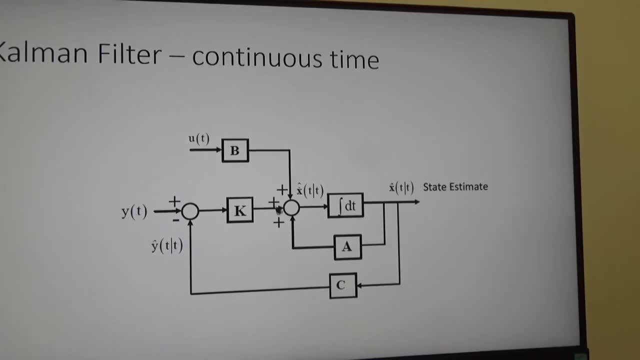 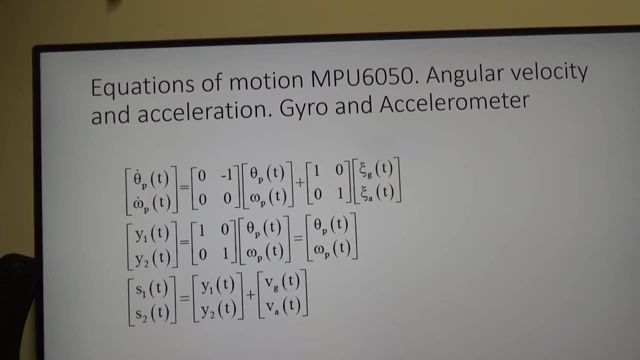 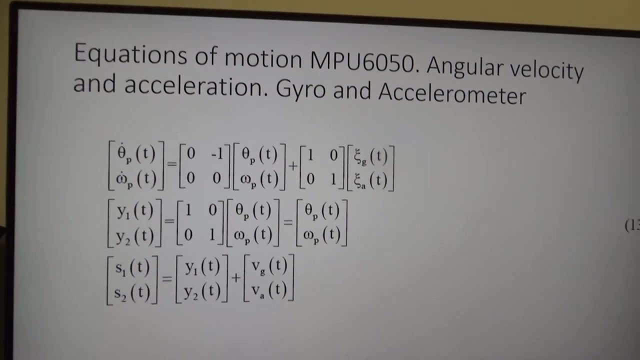 really not to need it. so we only need this part of the common filter now that this is it from my book and it's not the only way to do it. but these are the equations of motion, that's to say Newton's laws. in angular form, this is in: 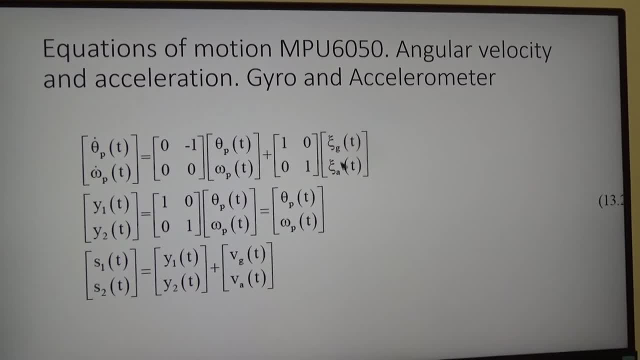 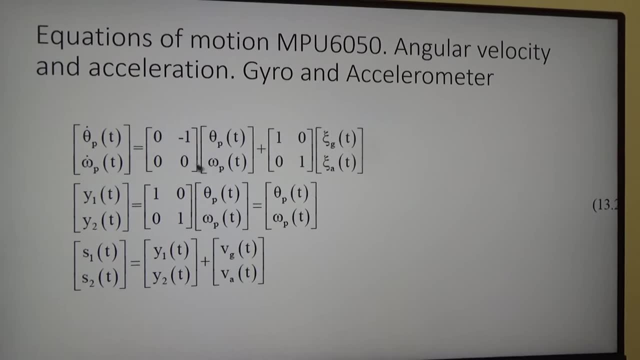 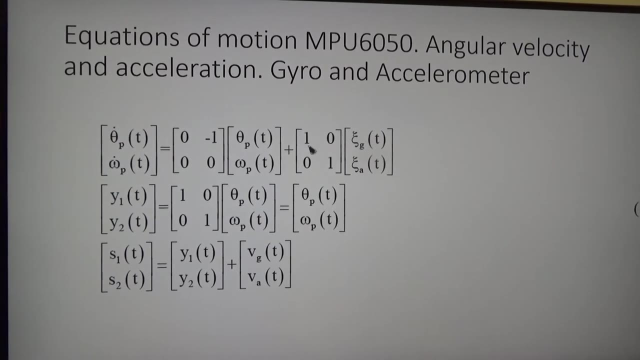 state space form. so this is like: X dot equals ax plus bu. you see, there's two inputs and they're both noise terms modeled as white and white noise. this is the a matrix. there's a negative there because, due to gravity going the other direction, this is just the identity matrix. I call that and call. 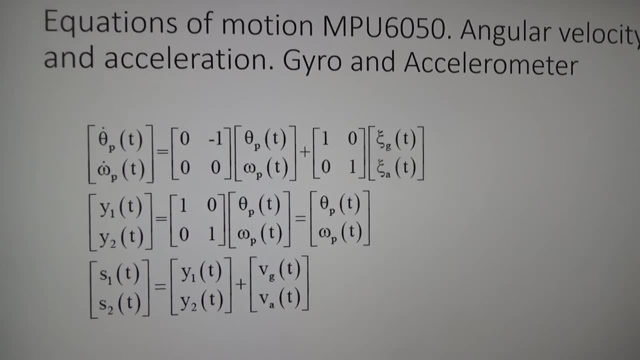 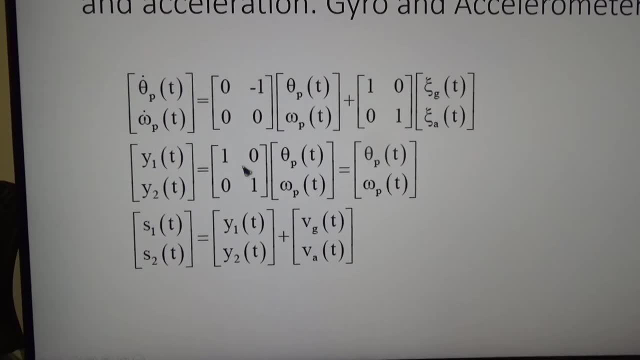 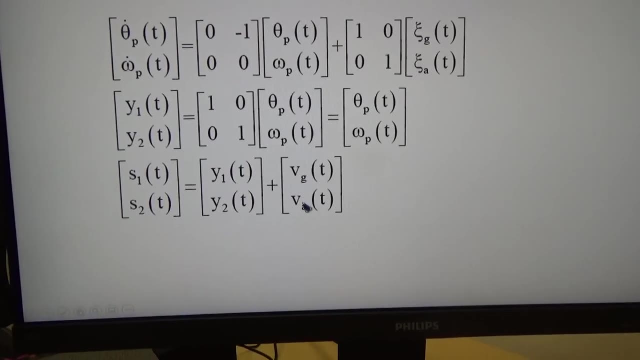 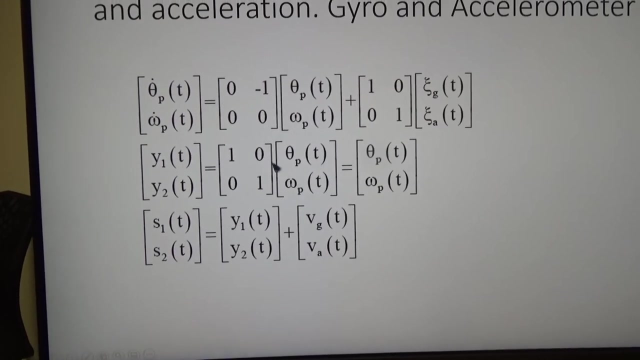 that D here, but to avoid confusion with the B matrix. and there's two outputs. again a vector, Michael C, X, C is also the entity matrix and to that there's measurement noise, here, VG and VA, and which gets added as a standard sort of equations for state space, and but just 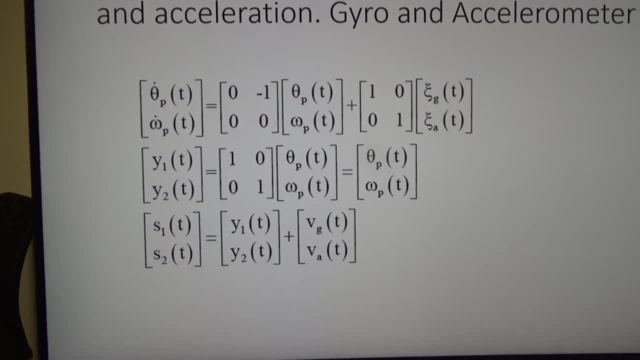 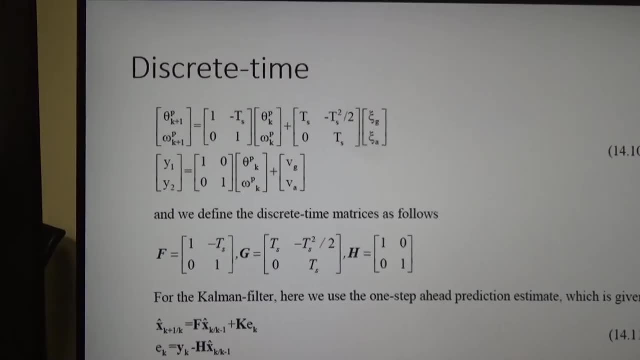 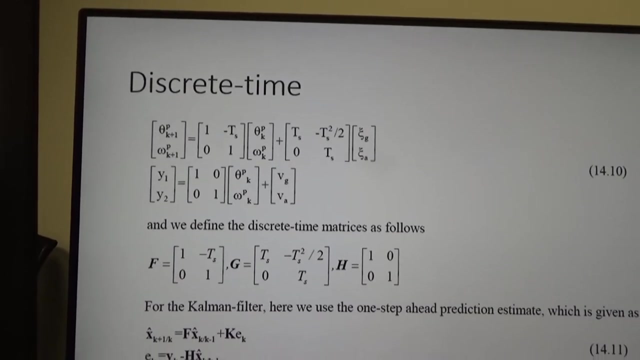 apply to the Newton's laws. so the first thing we need to do really is get them into discrete time for a particular sampling rate. now, the way that the, the Arduino works and the way this device works is it's not exactly galloping along in terms of measurements. I don't mean the ESP 32, but the 6050 and it's. 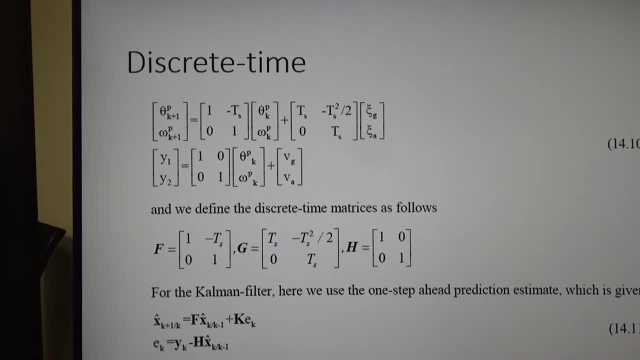 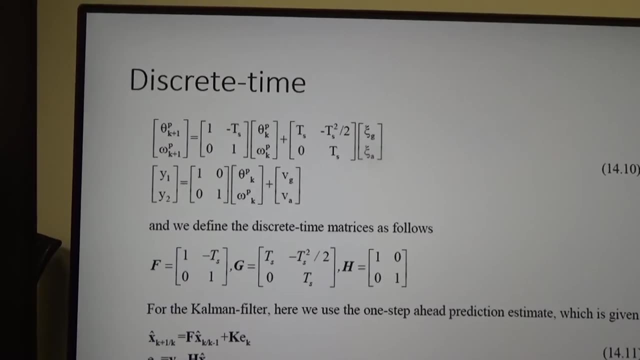 quite a slow device really, the way it's been set up with the libraries. I'm just using the libraries and so I'm quite restrictive for my sampling rate. I had to make it a hundred Hertz, but a hundred Hertz is okay for many things that are. 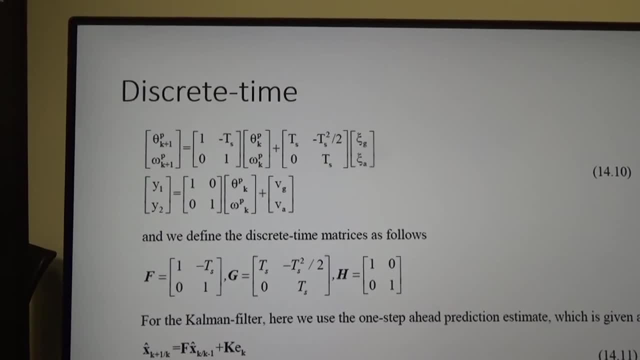 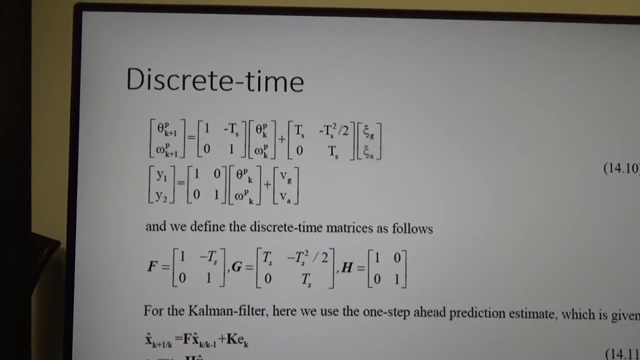 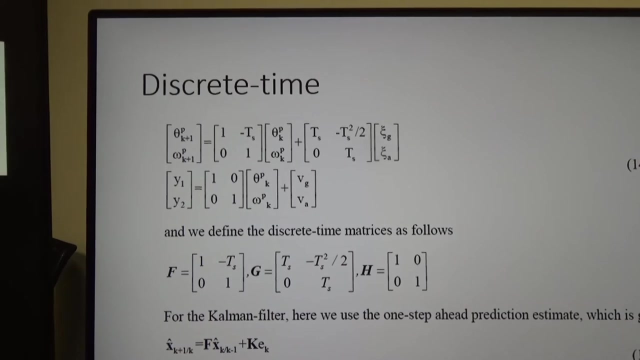 very slow and you know, like, like a sedgeway sampling rate of 100 Hertz is okay, because the bandwidth of the control system around that is maybe only a few Hertz. it's fast enough to keep it. keep it up upright when you discretize these and 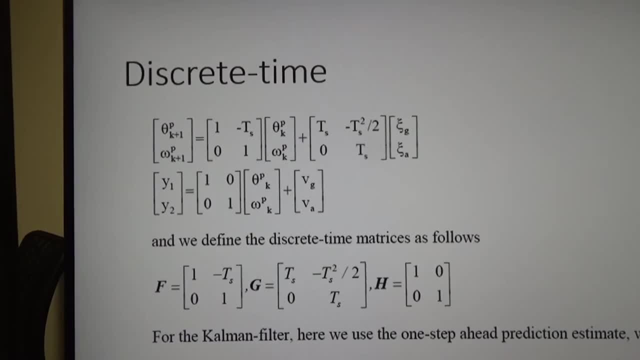 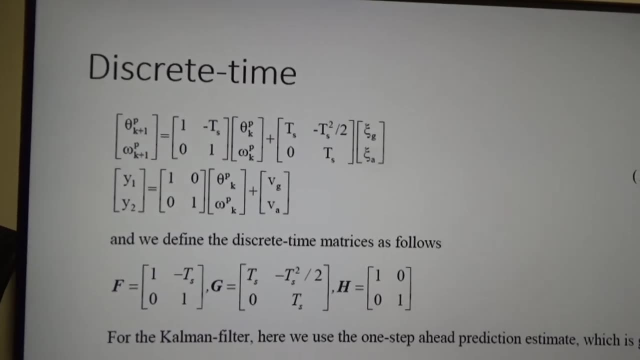 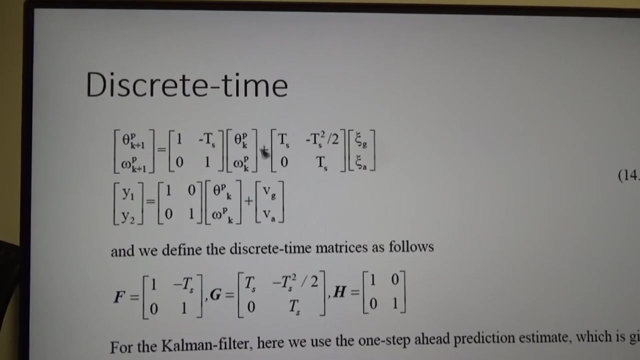 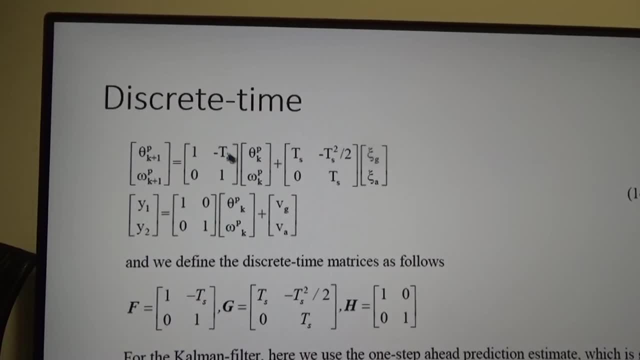 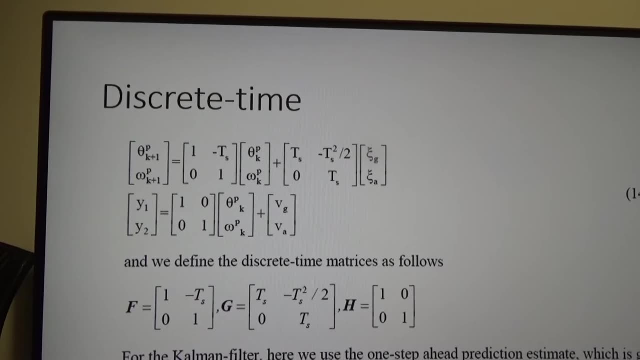 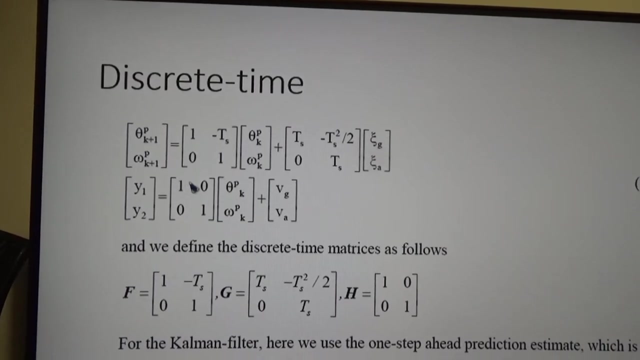 so it has to correspond- if you're doing it in real time anyway- to the real sample rate, otherwise it doesn't make any sense. if you're simulating just on a MATLAB or something, you could just put one in there for unity sampling. and then everything's respect to unity sampling, notice a C matrix. here is just the. 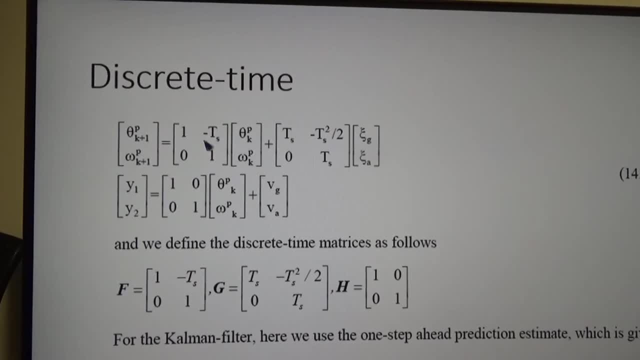 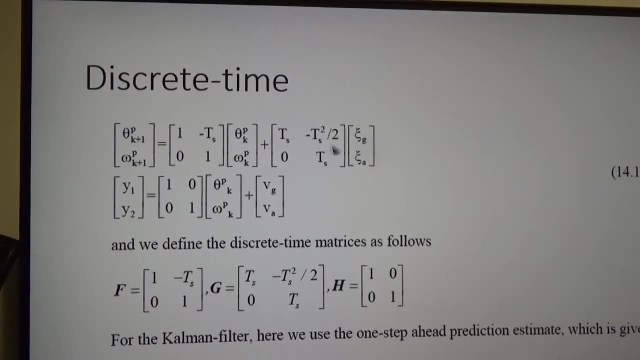 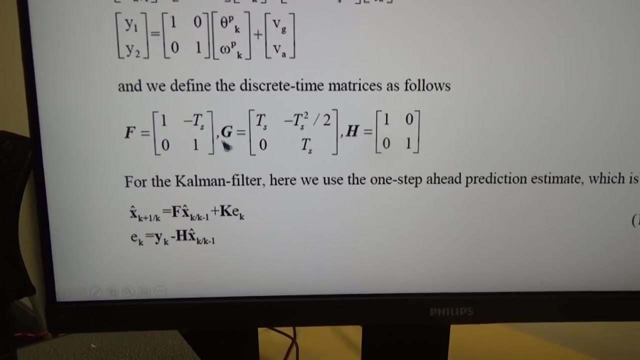 density, and these are the why I call this the F matrix and this I think I've called the D matrix. he could call it ge wanted to, so at least it's called that. Oh, it's called G here, I see, but in my program I've called it D, and that's the discrete version And the common. 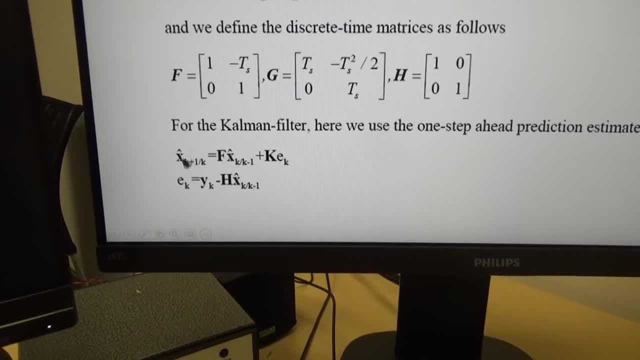 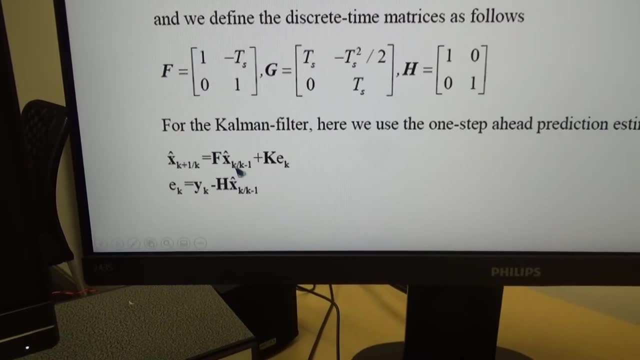 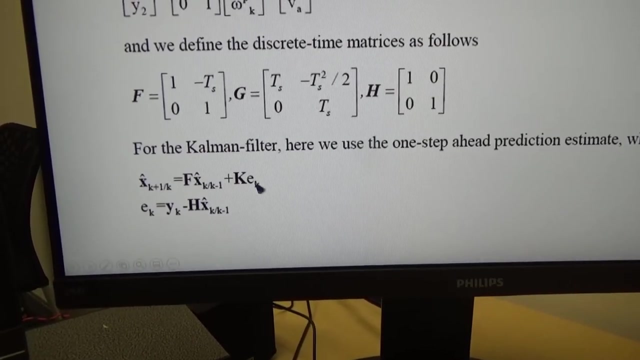 filter is just this iteration. here The hat, meaning the estimate time k plus 1 given k, is actually a predictor for one step. It's f hat k given k minus 1, plus this matrix K which we've got to find, times E, which is an error, and it's 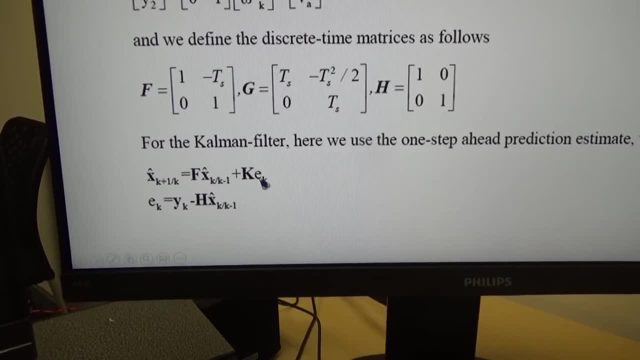 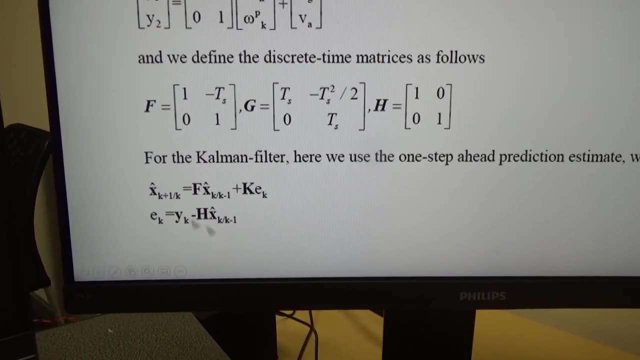 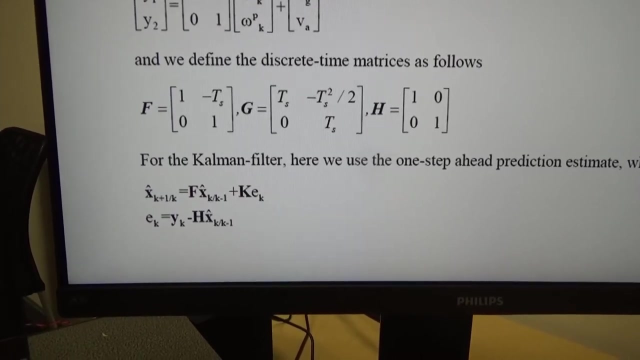 a vector, E is a vector error. in this case, Y minus H, X hat. that's the previous estimate And we just iterate that round, actually, or we can do it in a simpler form, which I'm going to implement. it We don't actually. 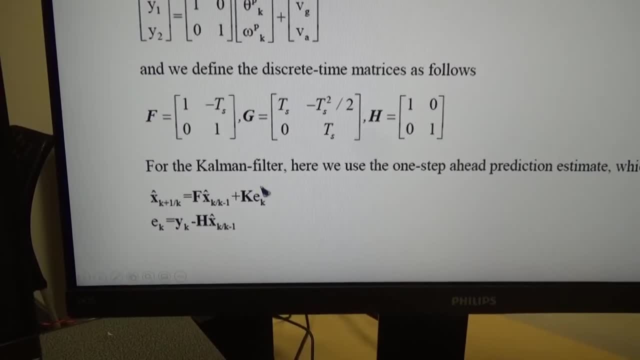 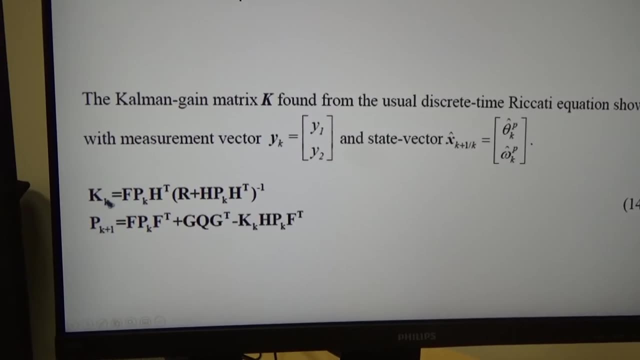 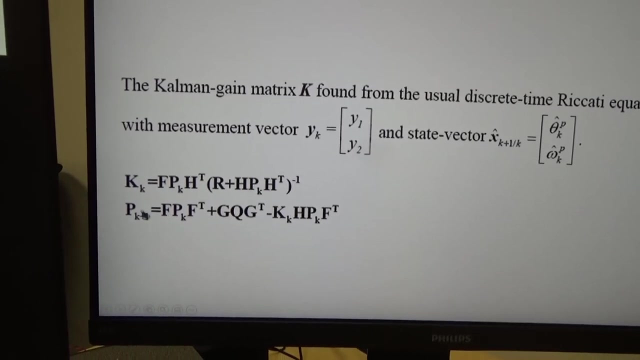 need the error. we can implement in closed form, closed loop form. So these are the equations that are called the Riccati equation. to find the Kalman gain matrix here We also need this other thing, which is the error covariance matrix. So you need to iterate that round, round and round and round. 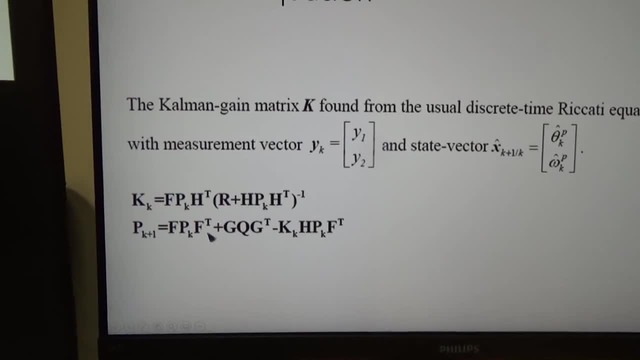 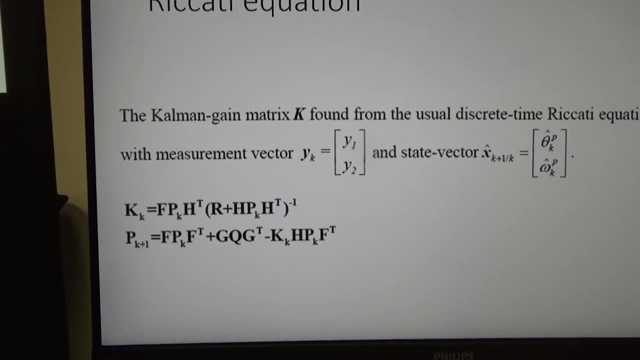 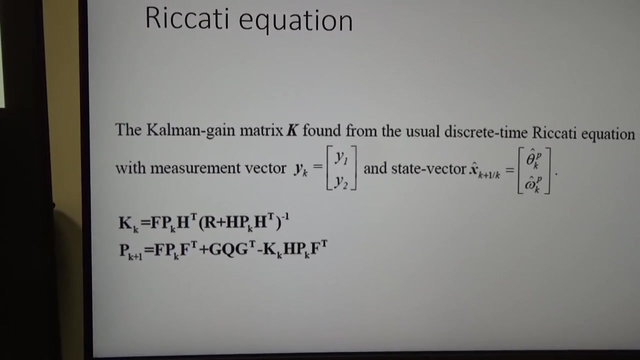 until it converges in steady state. Of course, if the matrices were changing with time, the Kalman filter can take account of that and then you'd have to iterate that in real time and it would track it. but you'd have to know the system varying in time, and to do that you often use an extended Kalman filter. 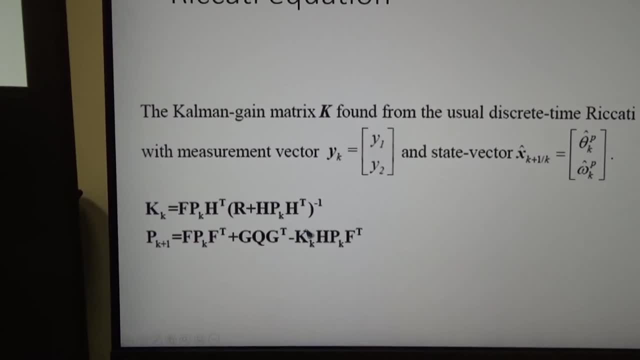 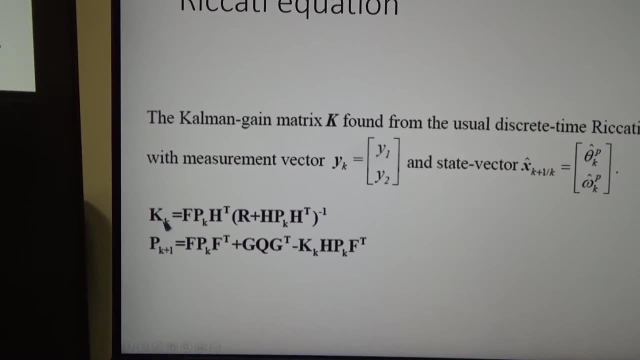 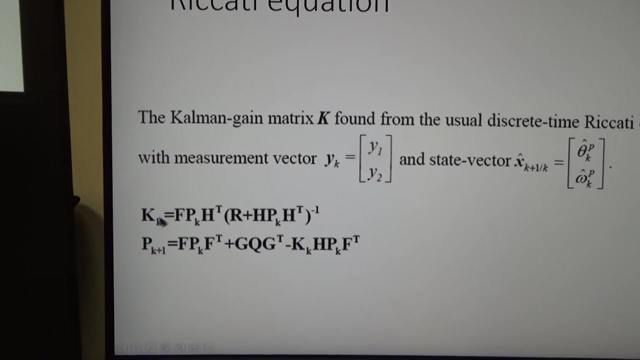 but that's not often guaranteed to converge, so there's problems there. But in this particular case everything's sort of static and we can iterate this equation and beforehand we can find the the gain matrix on MATLAB, which I'll show you in a minute. We need to know various things. Q- here is a matrix. 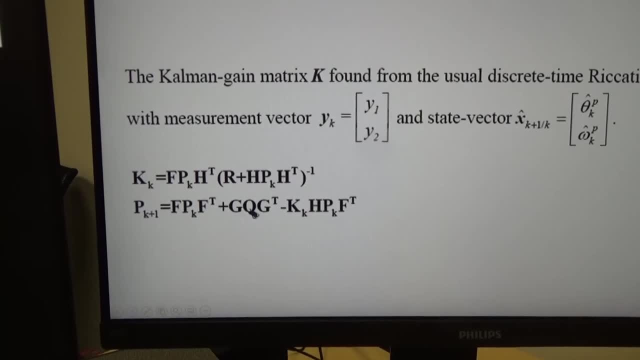 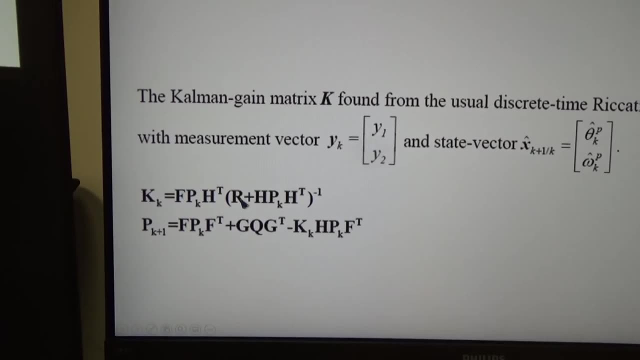 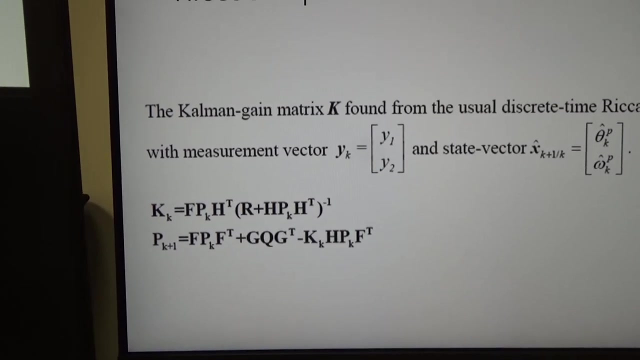 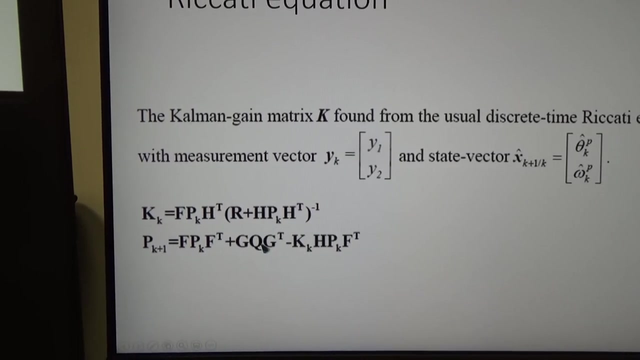 of the noise terms coming into the device, and R- here is the measurement noise covariance matrix. So these are also necessary for the calculation In MATLAB. it was just a one-line command to do it, but if you wanted to, you can iterate these round in MATLAB and in my book. I do this for a simpler case anyway, and you 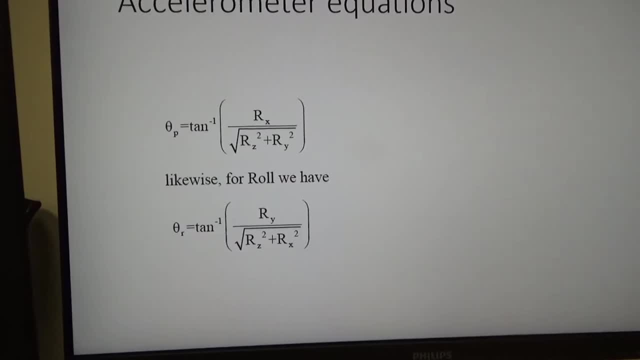 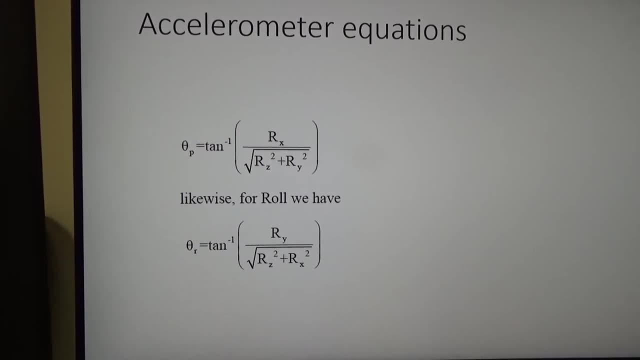 end up, of course, with the same answer as MATLAB anyway. So what's important here is that you need to know what the gain matrix is and what the noise terms are. So what I'm going to do is that the accelerometer actually gives you out the angle straight away, so you might think: well, what might what my even? 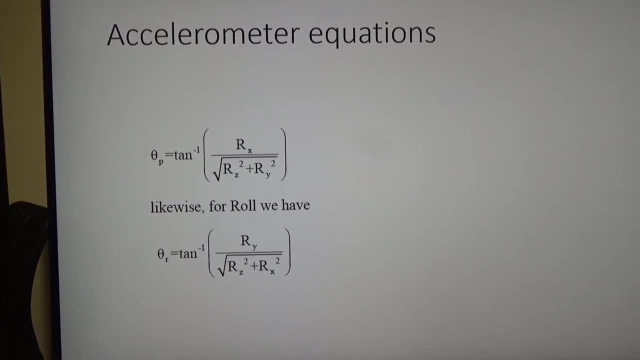 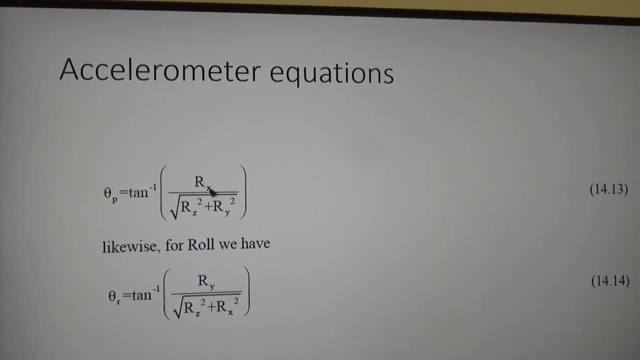 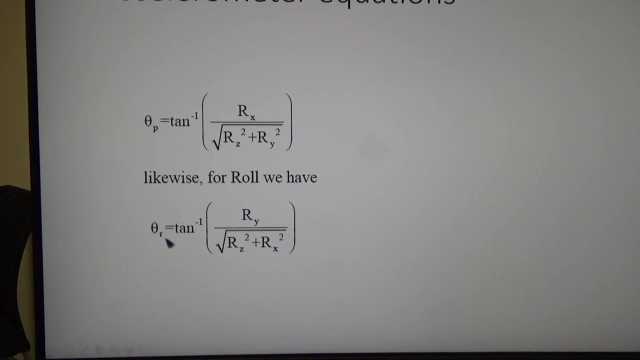 bothering, for if I can read the accelerometer equations, I can get the pitch and the roll straight off. I just need an arctan function here, which is that's the X reading of acceleration, that's the Z here and that's the Y, and that gives me the pitch angle, and I can do the same for the roll, but that's Y and 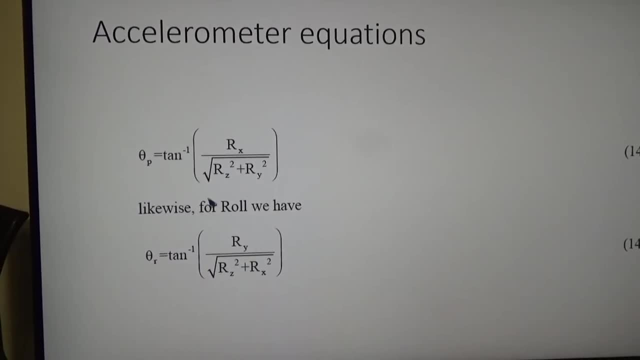 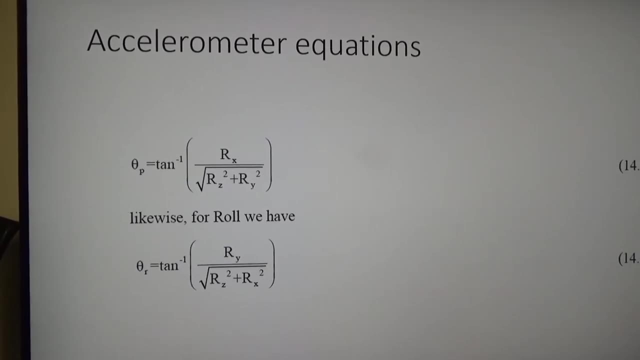 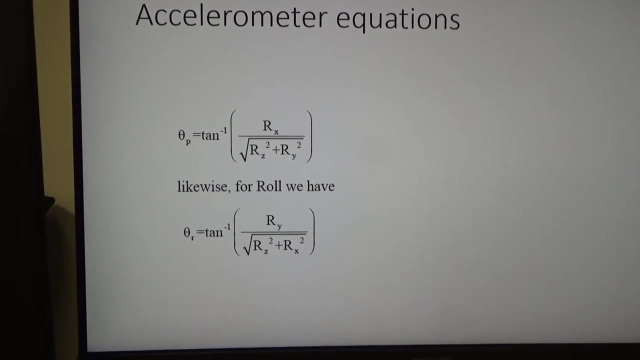 that gives me the pitch angle and I can do the same for the roll. but that's Y and the trouble with that is a little bit noisy. as I explained it. good at low frequencies, but not for fast, faster tracking, and I will show you a comparison of the two. but so the accelerometer, the reading that we get. 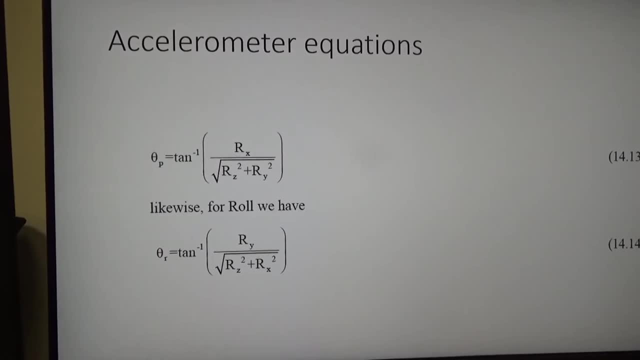 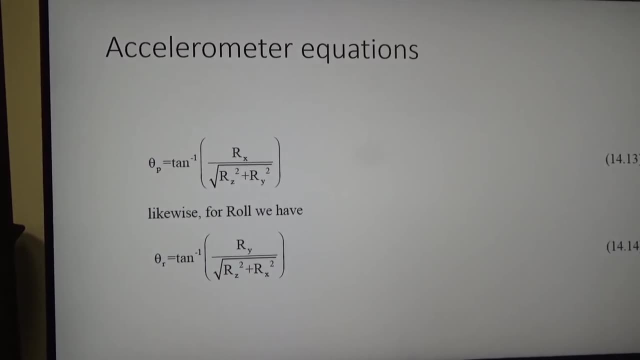 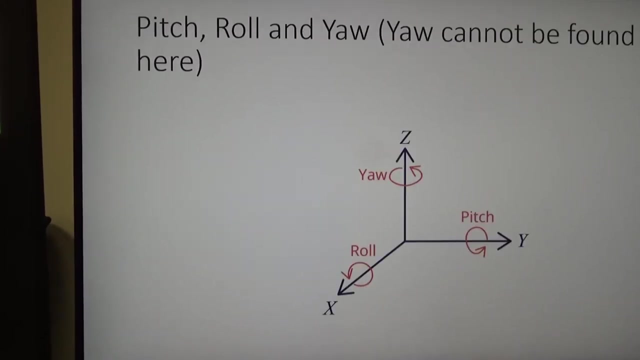 we're getting it isn't actually acceleration, it's an angle, so we've got to be careful there as well, although of course it does give off acceleration. but we're working out the direction which the acceleration occurs, which is a little bit different. So the definition here is roll, pitch and yaw, depending on. 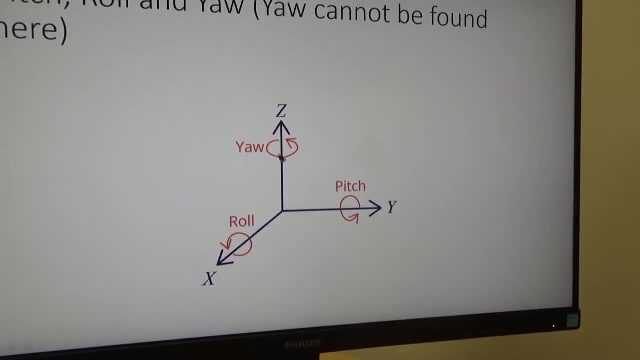 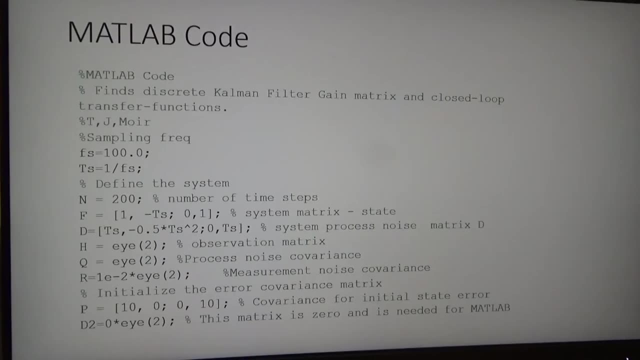 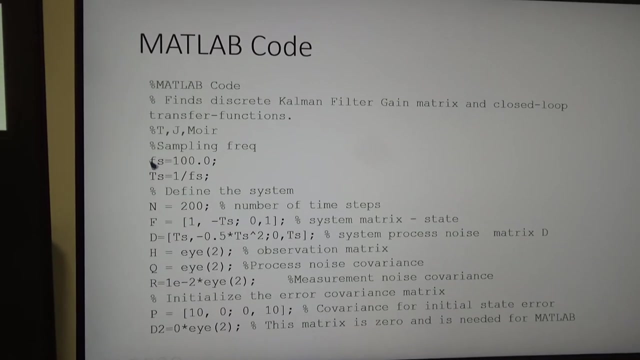 which way it's orientated. The yaw, as I say, we can't get because you need a compass, but we can get roll and pitch with a simple device. So the MATLAB code, so define the sampling frequency as- oh, I can't write on that- this is 100 Hertz, then there's a sampling interval. 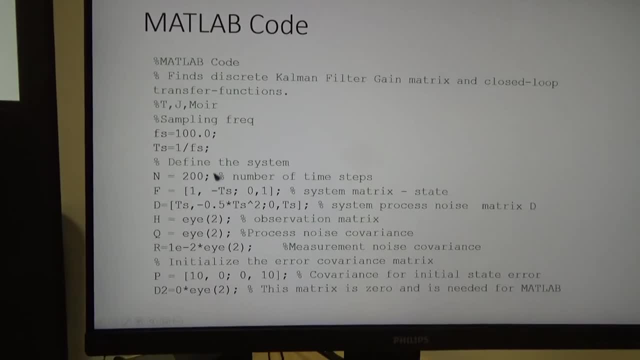 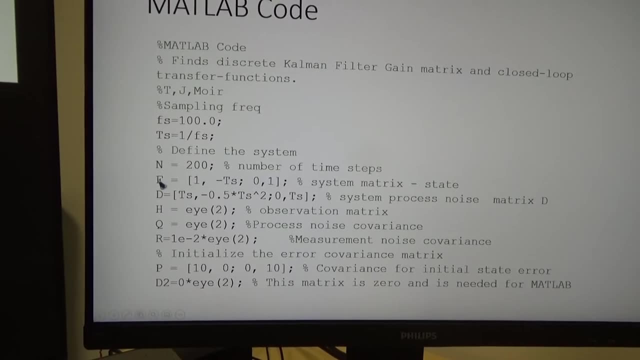 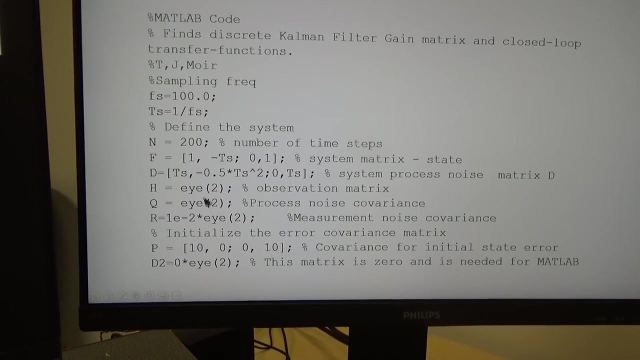 there's one over that, and then just sample for 200 points. don't really need that actually, that was for different simulation. then I define my F matrix, which was like the discrete A matrix, so my sampling interval and my observation matrix, which is the identity matrix, and I'm just making the 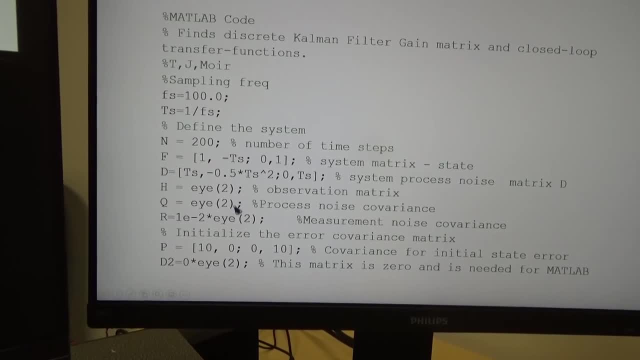 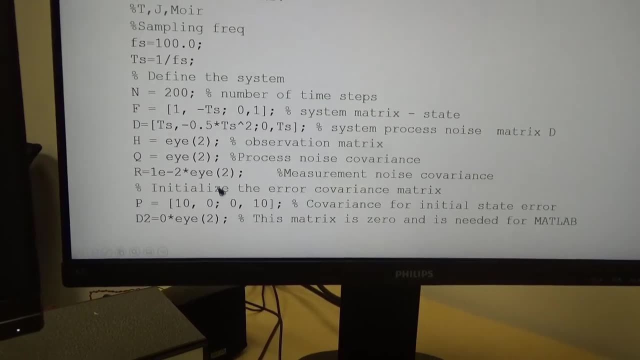 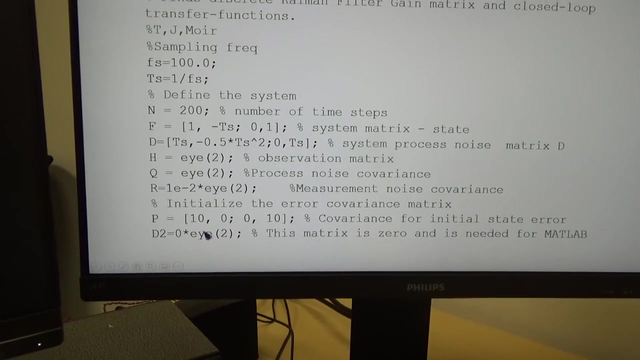 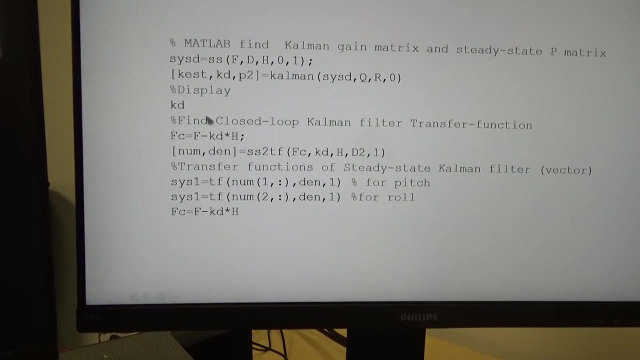 process, noise covariance unity and referencing the suspect to that. so I'm making the measurement. noise covariance is 10 to the minus 2. it's just arbitrarily at the moment initializing the error covariance matrix and I need another matrix which is zeros for the. that's just for the MATLAB program to run and on, and there's the. 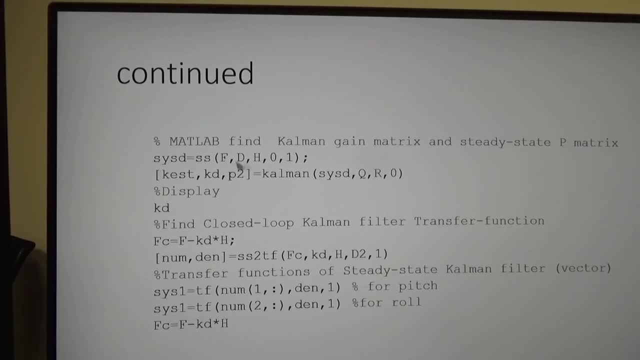 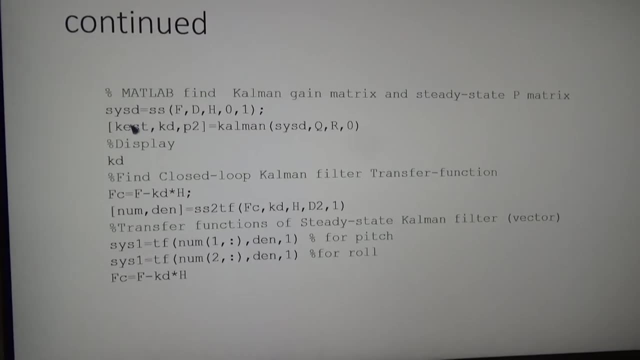 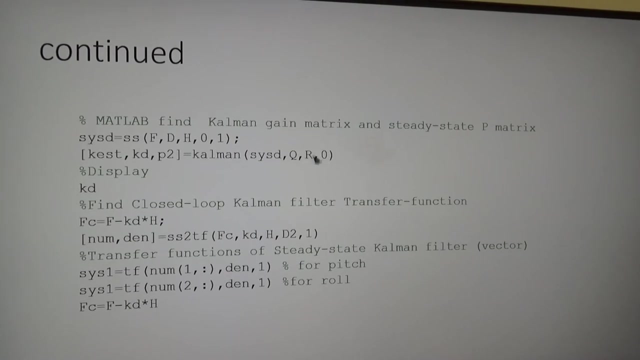 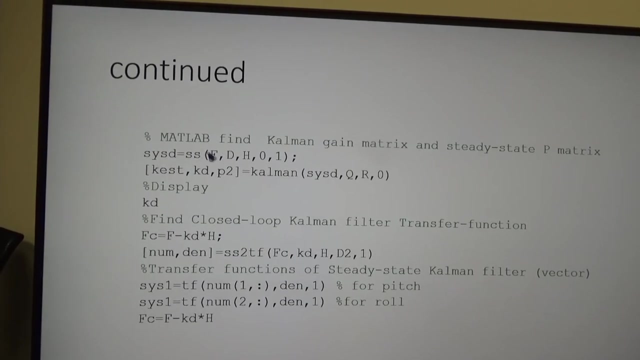 command and the one-lined function, if you like, in MATLAB. sorry, that's not. where is it? yeah, here, KS to KD keep: P2 equals Kalman and that's the system. Q and R, which is the noise covariances. that's the defining the system up here. 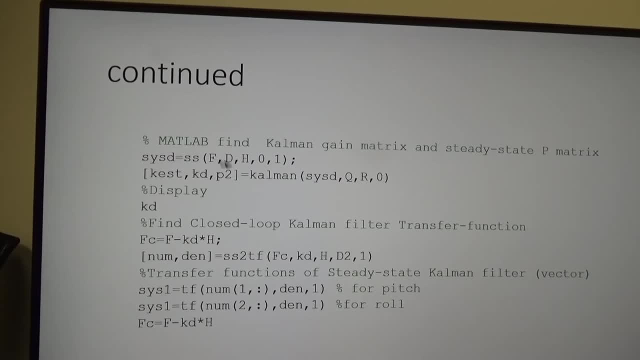 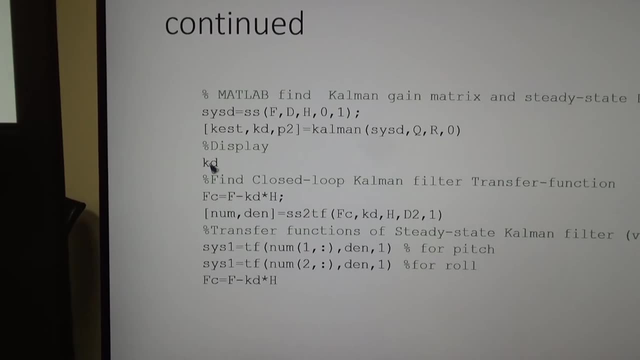 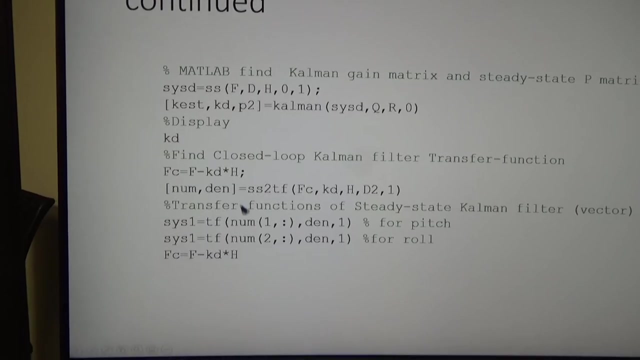 you're converting it from or defining it in state space from the matrices. okay, and then display KD, that's the common gain matrix and I use that in the program. and then I can find the closed-loop common filter transfer function if I want to, and really it isn't technically a common filter. this. 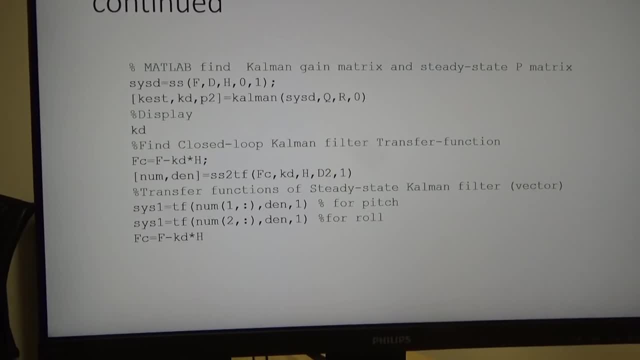 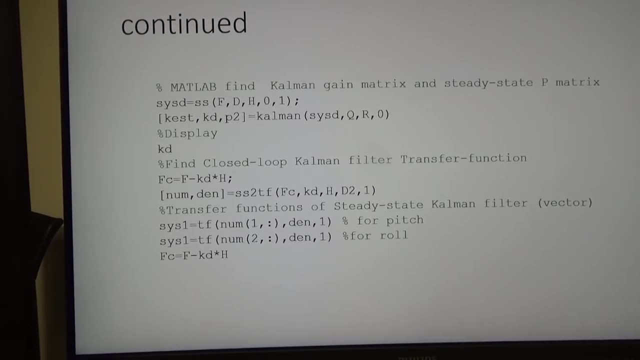 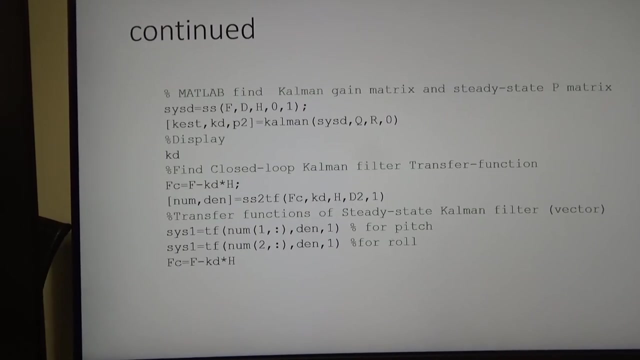 is a Wiener filter because it's a steady-state Kalman filter. however, Wiener never actually looked at state space. he only looked at transfer functions and he never even looked at discrete time. that was Kolmogorov, another engineer who looked at that. Wiener was a mathematician and, by the way, the 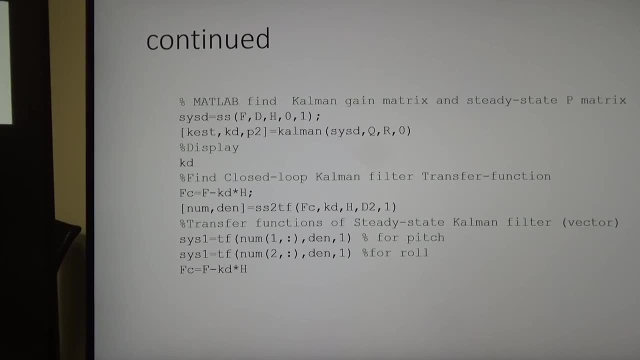 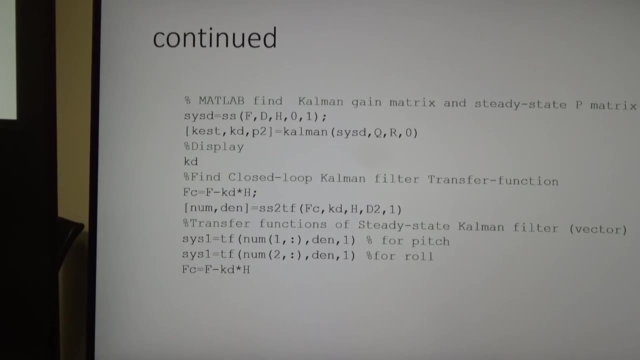 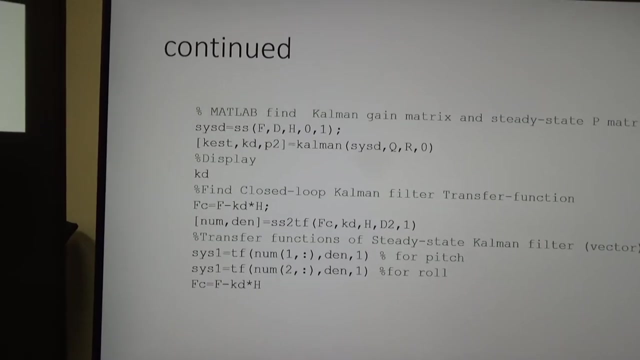 pronunciation of- because people have corrected me in the past- of Norbert Wiener is actually Wiener in the sense that he. that's how he pronounced his name. it wasn't Wiener, which is the German term, that was translation. it was Wiener was how he liked his name to be told, and I know that because a colleague 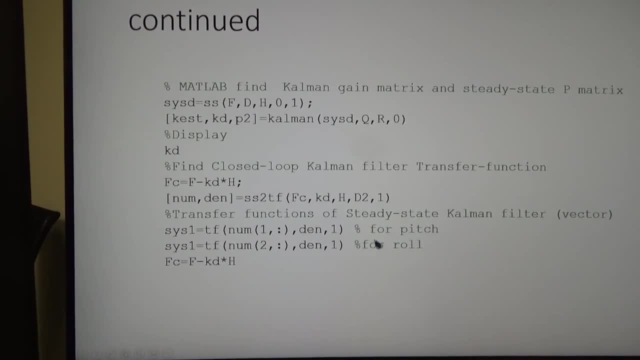 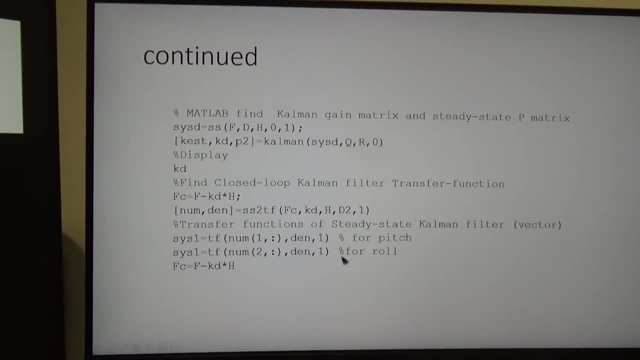 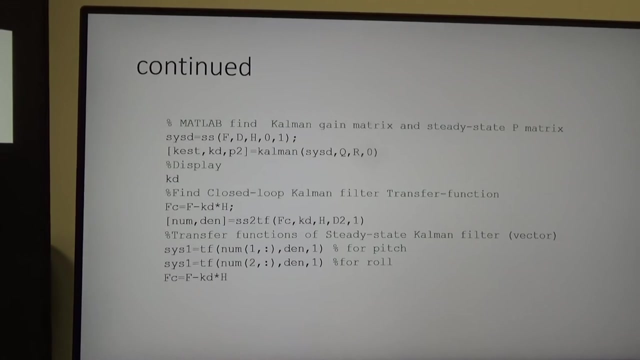 of mine old friend worked with him way, way back in the 1960s so when he was in America. so that's how he got his name: Wiener. he pronounced his name. so it is really a steady-state. Kalman filter is actually a Wiener filter and I'll show you you can get the transfer functions for them for. 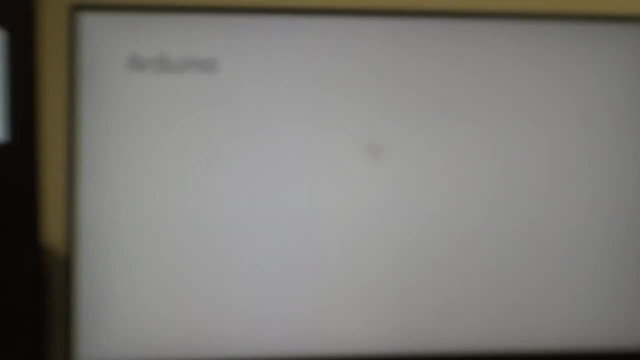 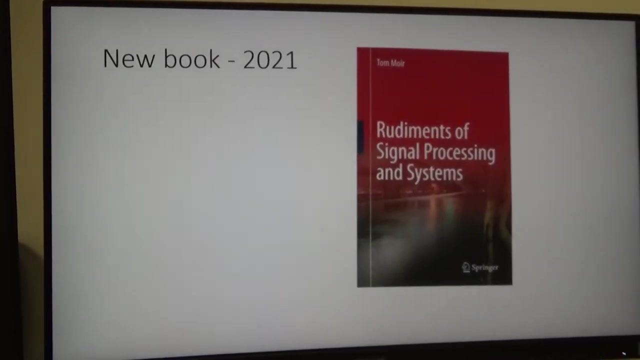 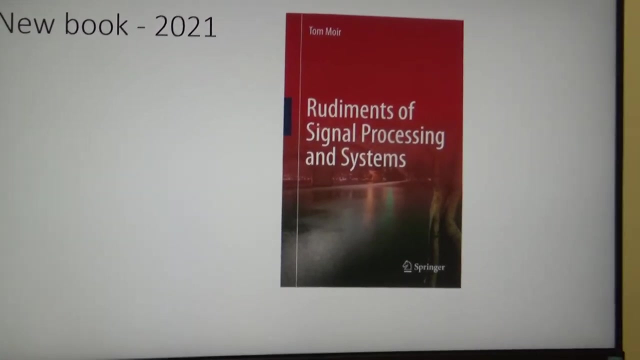 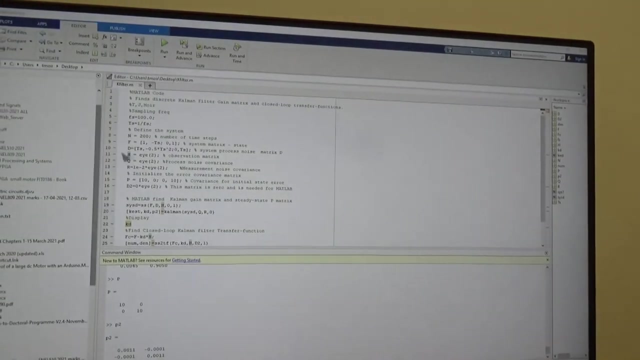 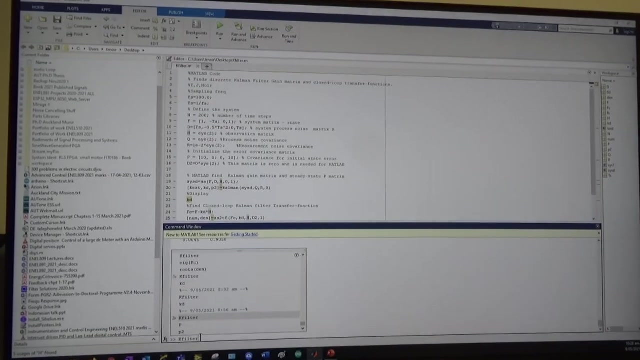 that particular sampling rate. so the Arduino stuff I'll come to in a second. I just wanted to say this is my other book which is coming out this this year: rudiments of signal processing and systems. that'll be out hopefully in 20, 2021. so back to the is the MATLAB code here and I'm just going to run it and you'll. 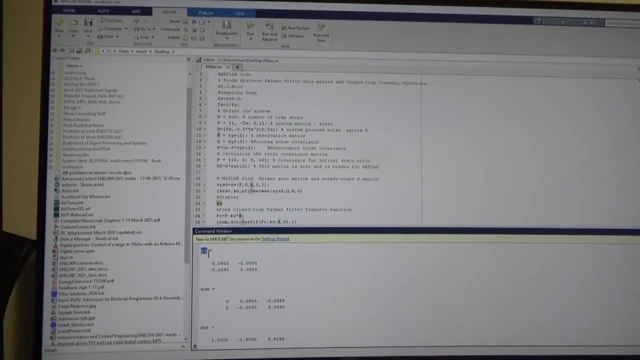 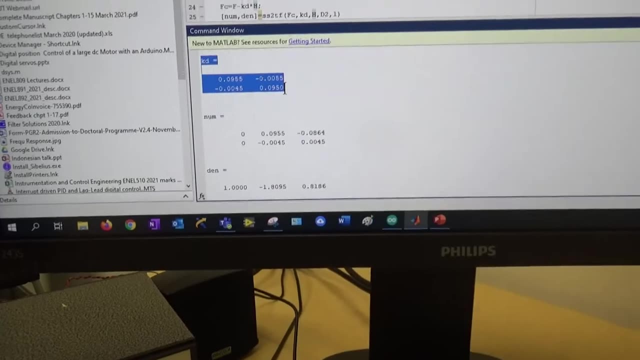 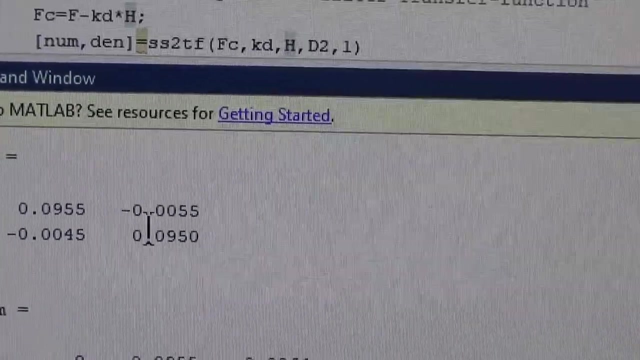 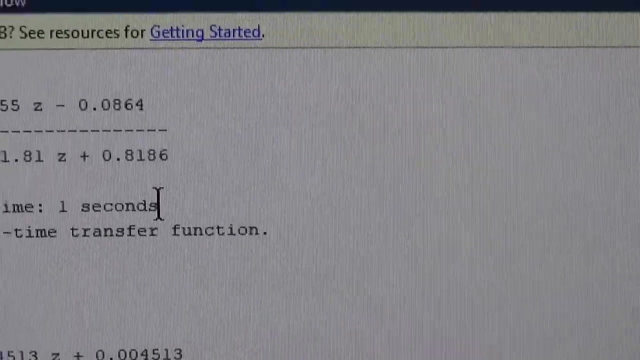 see, gives out. there's the matrix of gain, so you can see that, yeah, zero nine five minus point zero, zero, five, five, and so on. and we can also find the transfer functions, because there's two, because it's multi variable and it works out. these are the transfer functions of the column with the filter, so you could. 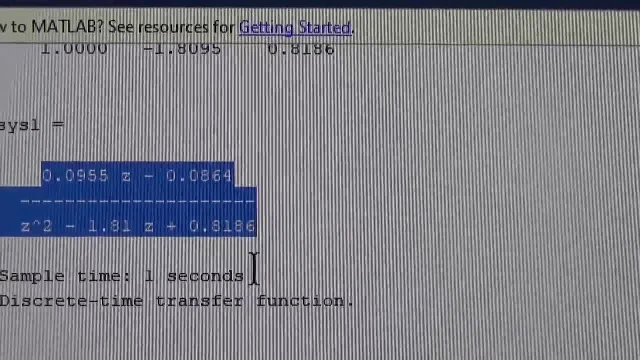 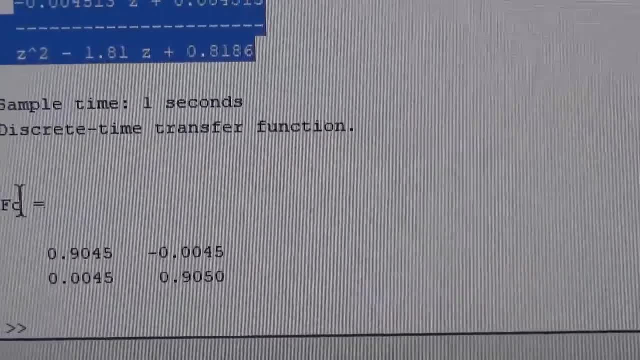 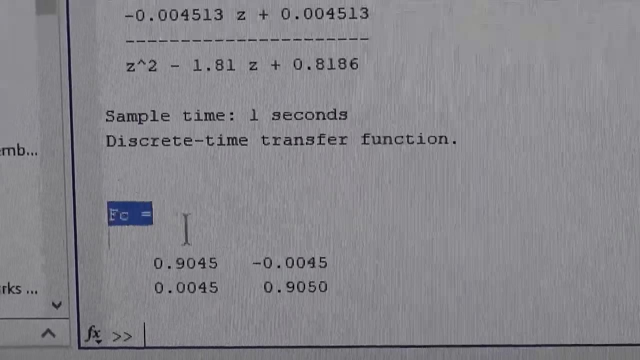 actually implement them as well, rather than implementing the in state space format. that's another alternative- should get exactly the same answer in this case. that's the closed loop, a matrix or F matrix. here you can work out its eigenvalues and you'll see that this is the same as the matrix for the filter, so we can get that in the next slide. 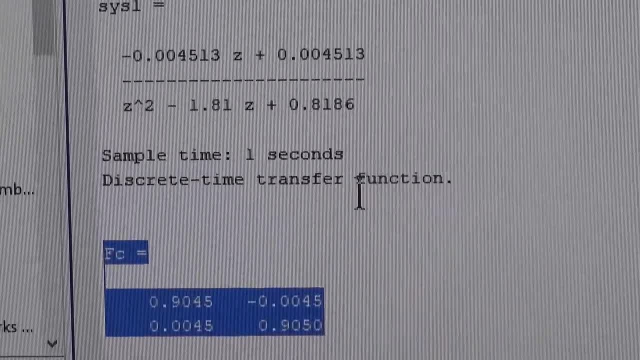 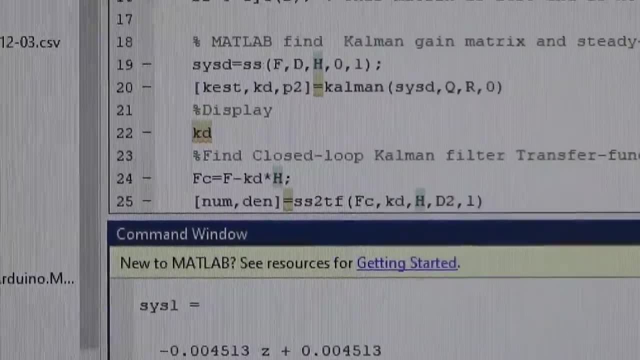 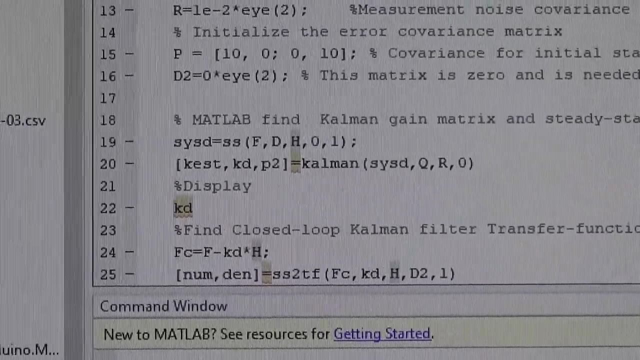 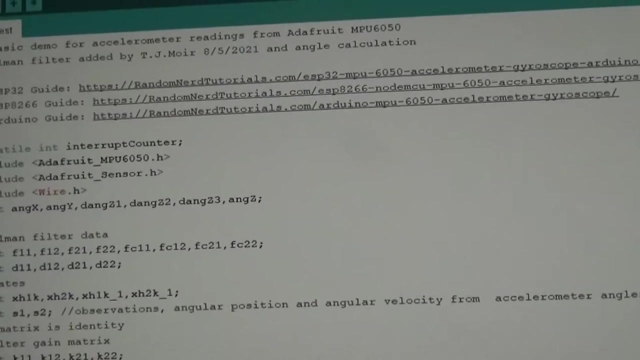 eigenvalues of the poles of the closed-loop Kalman filter, which are also the same as the roots of this polynomial here. so let's go to the Arduino and fire it up. so I'm just going to here. it is here. so so a lot of this I took from the 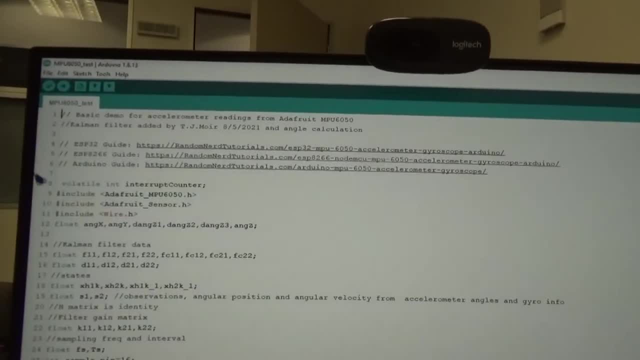 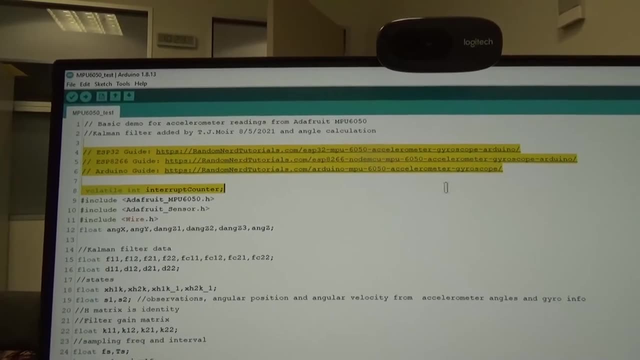 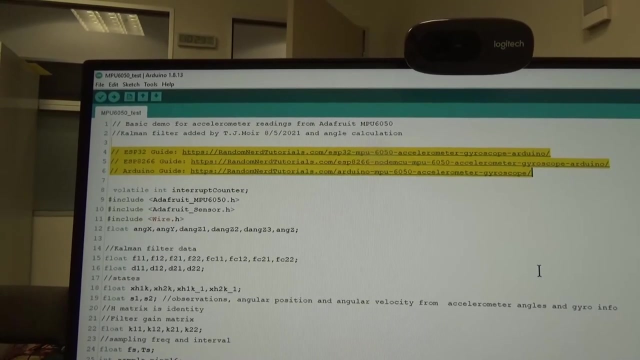 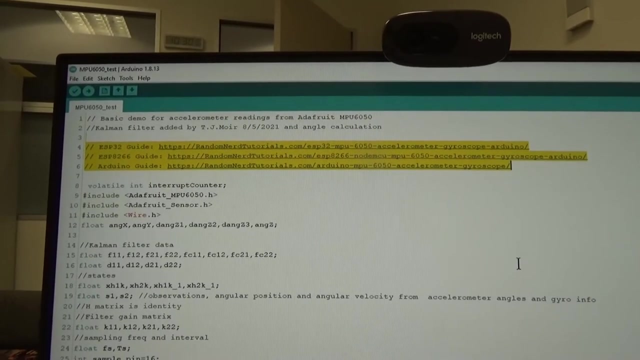 random nerd tutorials on these websites here and they're pretty good. so I've, you know, obviously acknowledged that. but I noticed they didn't put the calculations with the arctan in there, so they were just giving out the raw accelerometer and accelerometer and gyro data and I really wanted the angle as 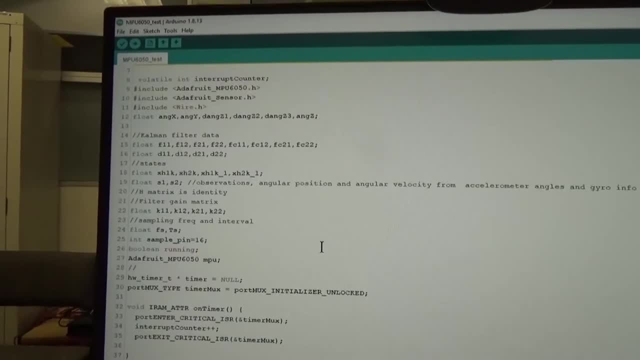 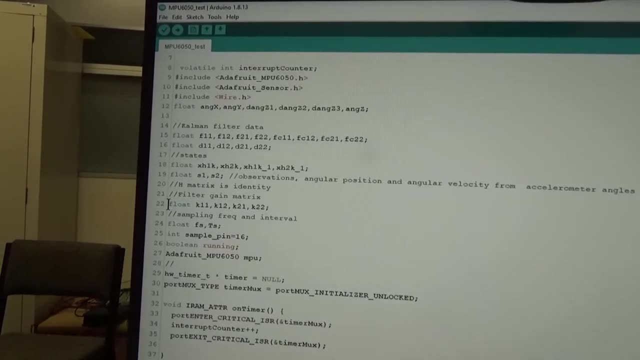 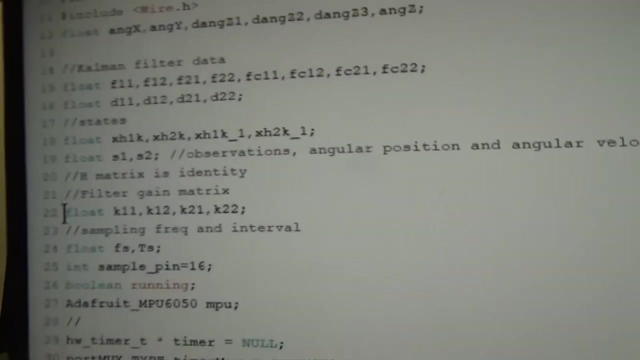 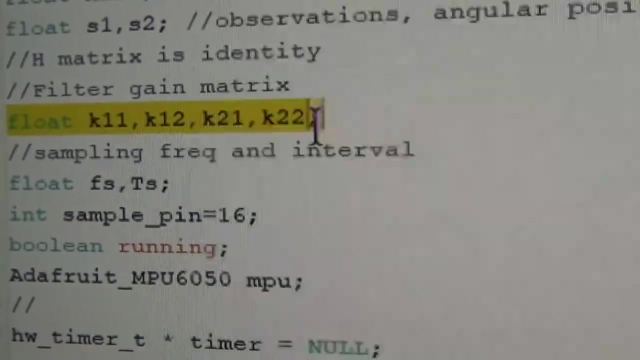 well. so I just stick that in as well, plus the Kalman filter, plus I use interrupts for the sampling frequency. you'll see here the Kalman gain. I'll just put my glasses on so I can see what I'm doing. yeah, here the Kalman gain in terms of the, because we don't have matrices here, we just have. 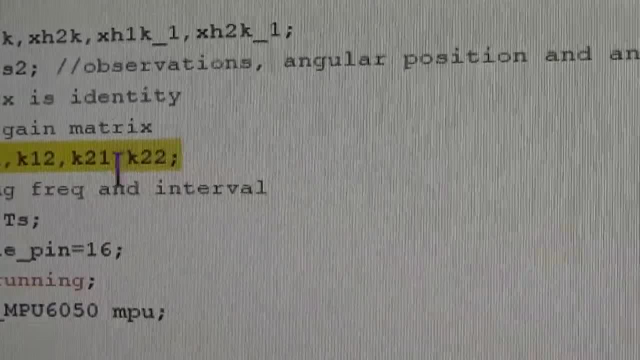 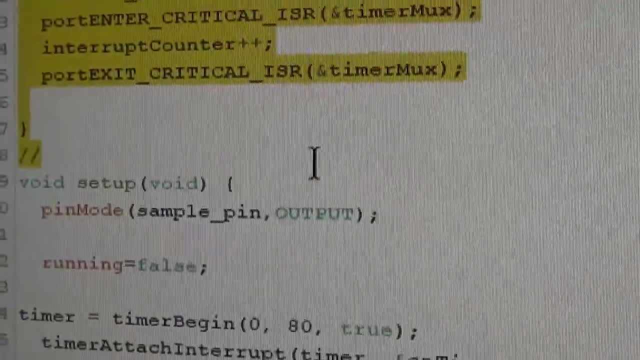 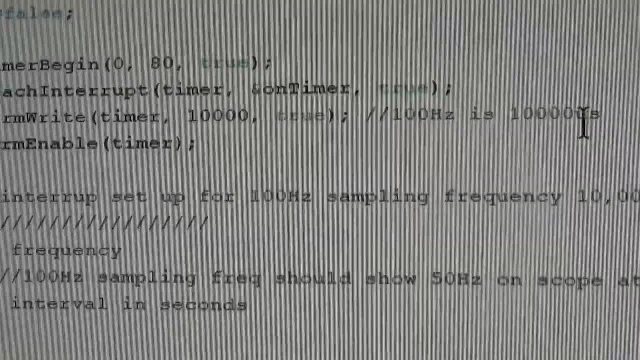 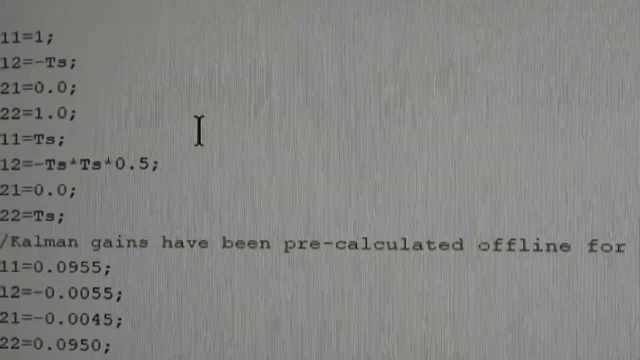 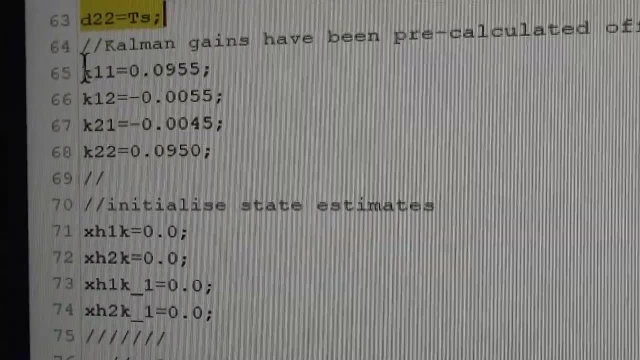 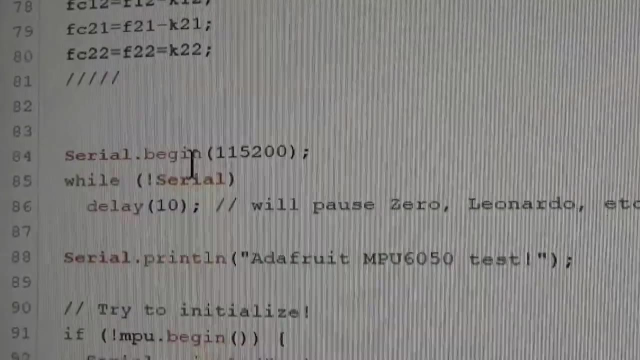 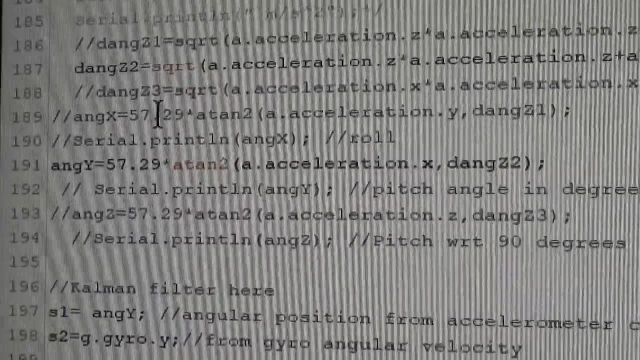 100 Hertz. and this is me setting up the F matrix for the Kalman filter. and then I'm just typed in the K values I got from MATLAB and these initial state estimates and if we go down to the actual calculations, you see that you have to have the square root of the Z. 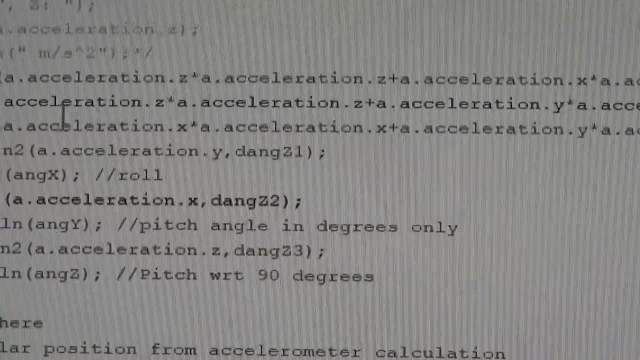 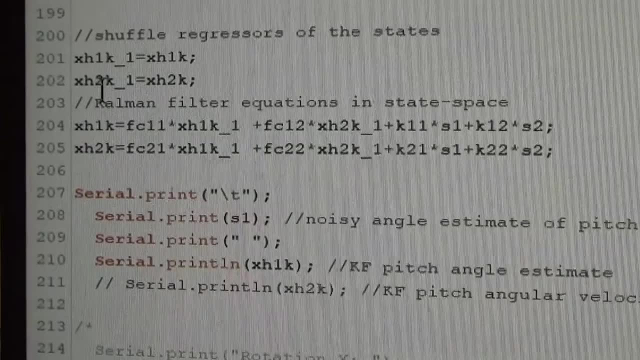 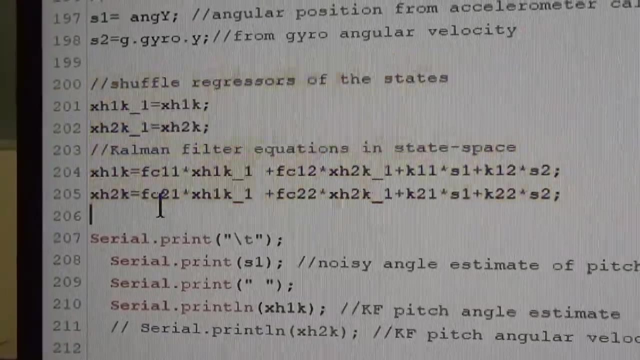 squared plus X plus Y squared part and the arctan function to get the angle. then the Kalman filter itself is isn't too complicated because it's a steady state Kalman filter. it's just the matrix form. I've had to put it into long hand. 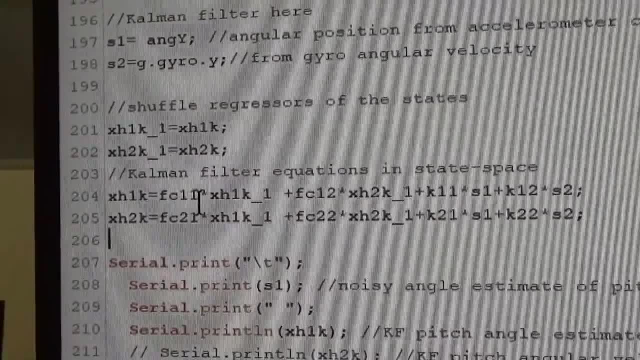 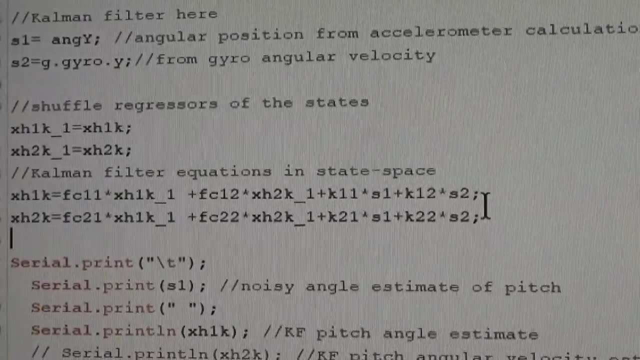 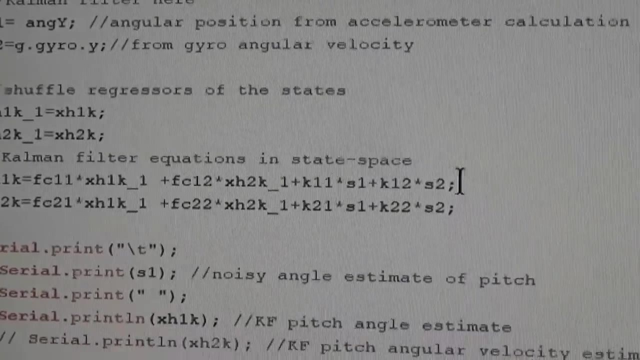 form: X hat 1 K equals FC 1: 1 times X hat 1 K minus 1 plus and so on, where s 1 and s 2 are the observations, and that's case it's the acceleration and gyro readings and I just going to use, I mean 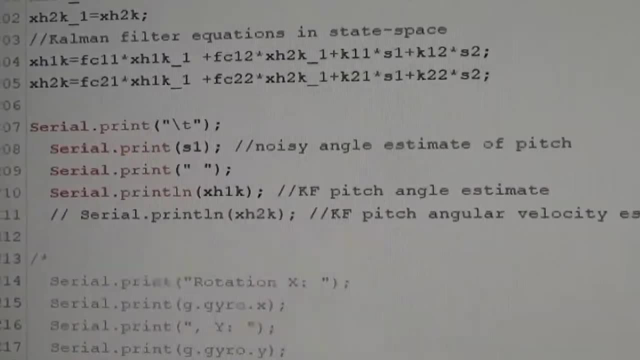 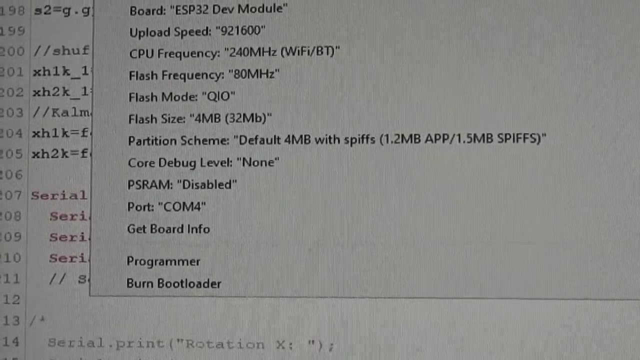 I know it's very crude but I'm just going to use the serial print, and which means I can actually use this serial plotter to put the two values. so I'm. what I'm going to plot is the roll accelerometer angle and the Kalman filtered one, and here it is. here i'm just going to take the. 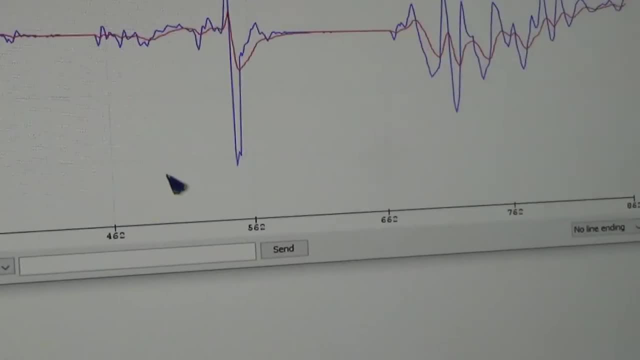 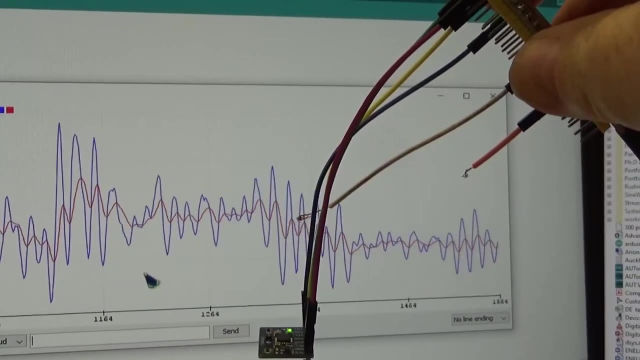 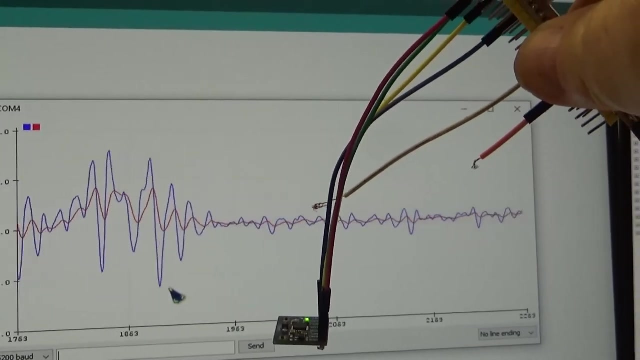 this off the scope so that i can show you so sort of in front of me now. so the red one is the Kalman filter output, you see, the smoother one and the- if i sort of shake it about a bit. and the blue one is the accelerometer reading as it comes out and as i tilt it, you see. 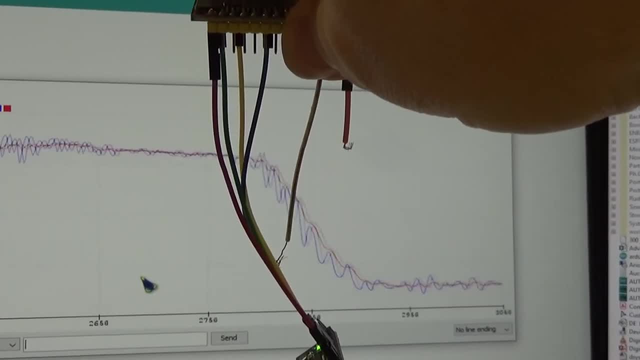 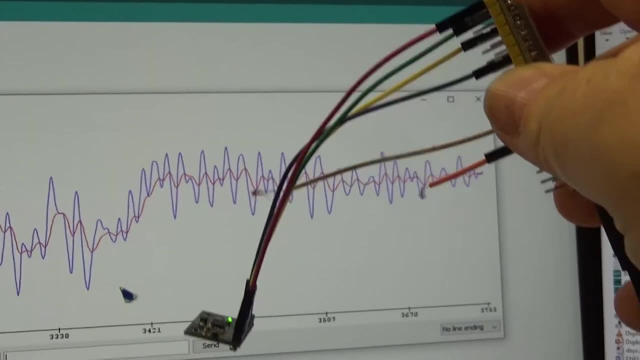 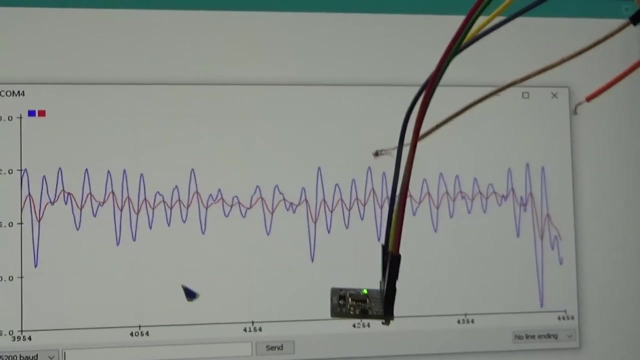 it's going up down measuring the angle. okay, so this is using. so this is sensor fusion. it's it's taking account of the accelerometer as well. the Kalman filter estimate is at least the blue one is just the accelerometer readings on their own. now, as i said, the accelerometer doesn't. 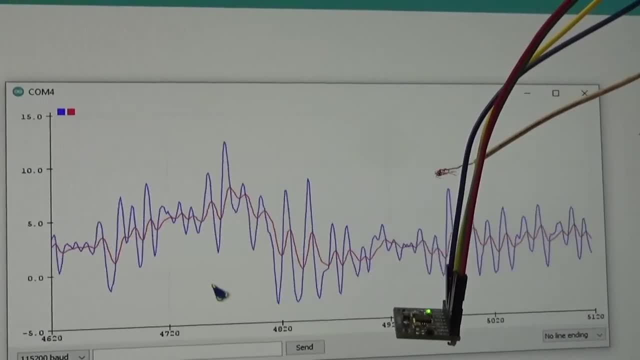 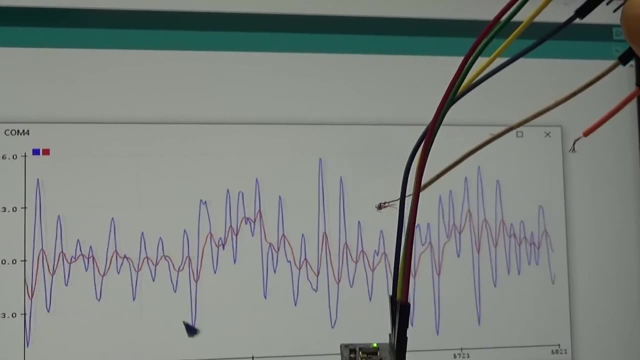 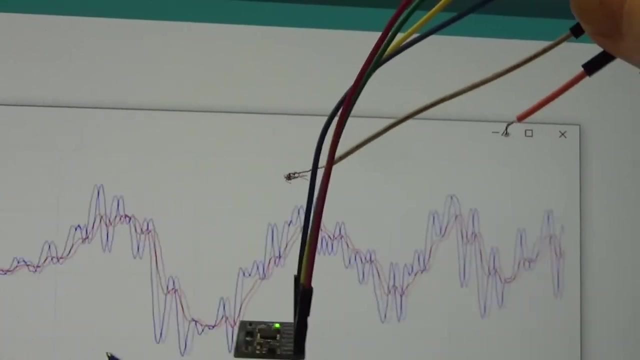 need to be integrated because it's a direction, so it's found from the arctan function. you don't integrate acceleration twice to get that angle, you just work out an arctan function and there it is really a real-time Kalman filter- not exactly super fast.